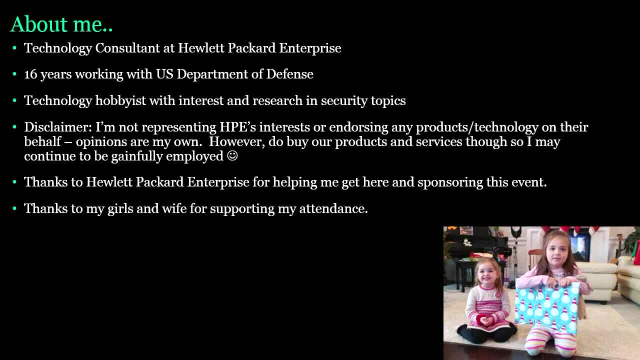 Anything from system administration early on to software design and development and systems engineering. So a little bit of a handyman I guess, which is something I guess we all kind of need to be these days, especially in terms of development, where we have so many security threats that can. 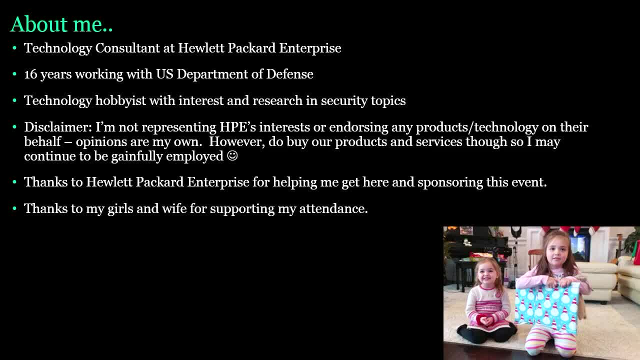 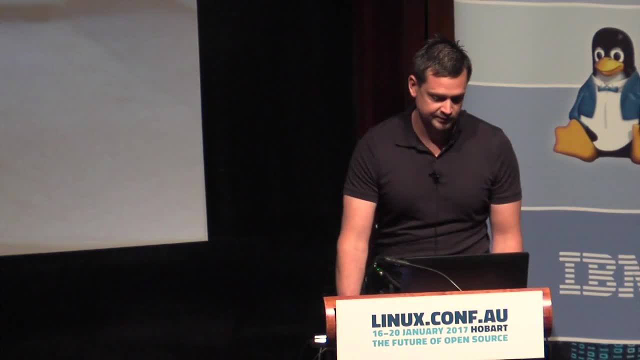 be dealt with at the application layer if we understand how to do so, And that involves being a little bit of a jack-of-all-trades in the cyber realm and the development realm, And thanks to Hewlett-Packard for sponsoring and helping me get here- And I'm not representing them. 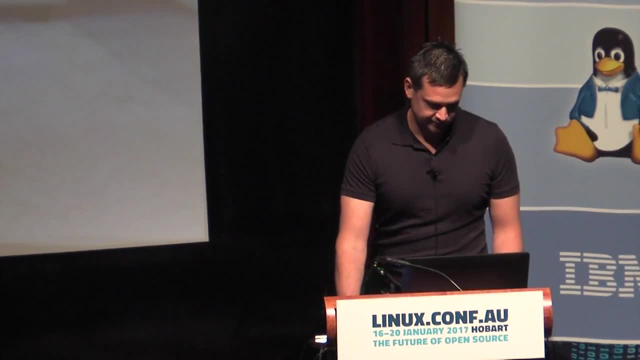 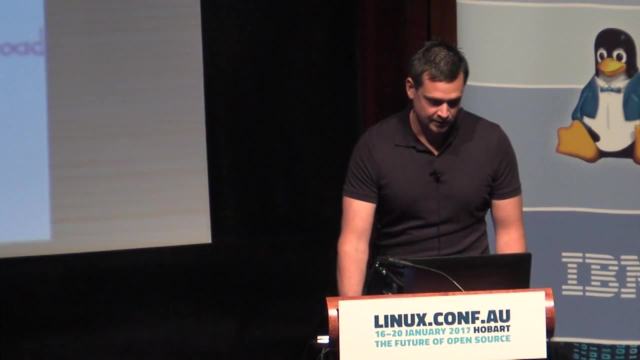 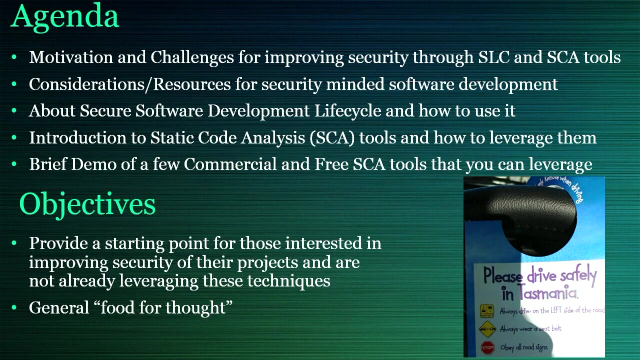 necessarily their products or anything, but certainly buy their servers if you like them. And thanks most importantly to my wife and my kids for letting me get out here. So quick agenda. This is a real big topic. You can find talks, papers, entire text dedicated to every. 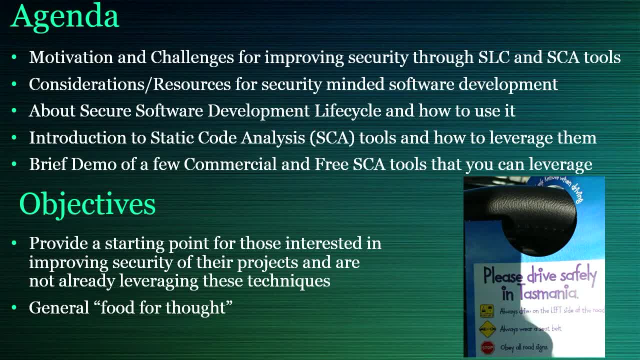 aspect of this. So we can't really get too deep in a 30-minute talk, but kind of give you a general overview of static code analysis and how it fits into an overall secure software development lifecycle, Because you really need to make use of both tools and also an architectural approach to security, to 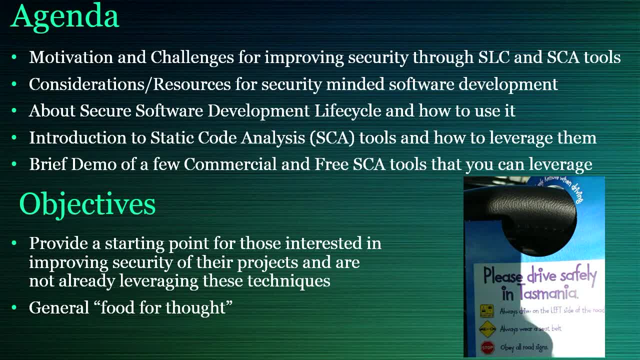 make more secure code, And it really points to provide a starting point for those interested in improving security of their projects, if they're not already leveraging these techniques, Or also for anybody that's maybe just getting out of school or getting into programming and really haven't given these. 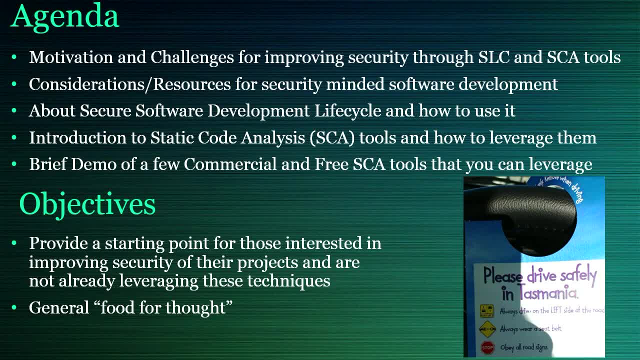 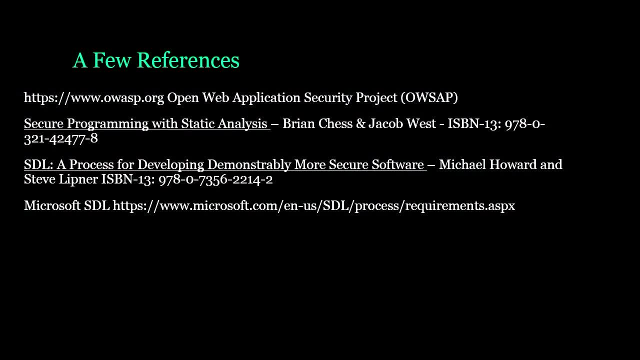 things, a lot of thought And, just in general, a few for thought. of course, Before I even start, there's a couple resources you should definitely consider looking at, if you haven't already. Number one for the open source community would be the web application security project. 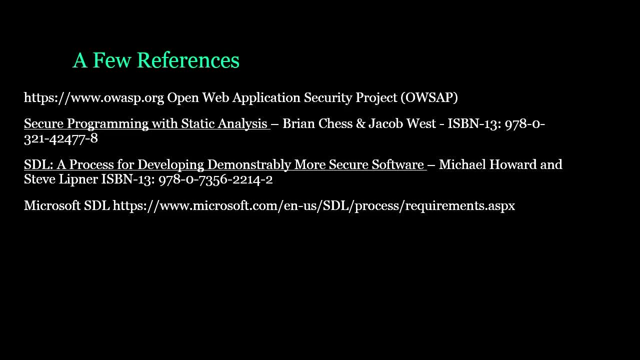 It's got a lot of great information. I certainly borrowed a lot of their diagrams for this. If you're interested in some of the technical details of how static code analysis works, it's a pretty good book. It's a couple years old. It's by some of the guys that created Fortify And, in regards to the security, 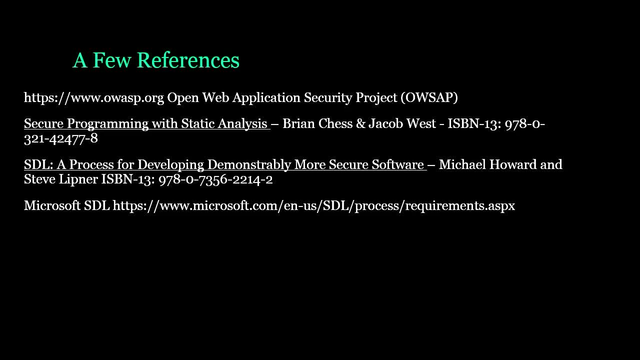 development lifecycle. there's a lot of books out there. This one is by a guy from Microsoft that helped implement it there, And certainly Microsoft's website. they were one of the kind of companies that really kind of started driving the idea of developing a formal model for security. 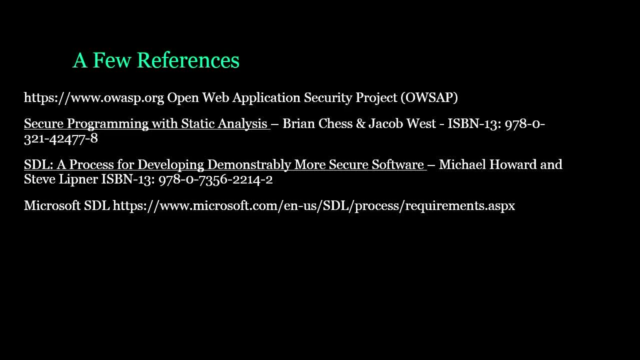 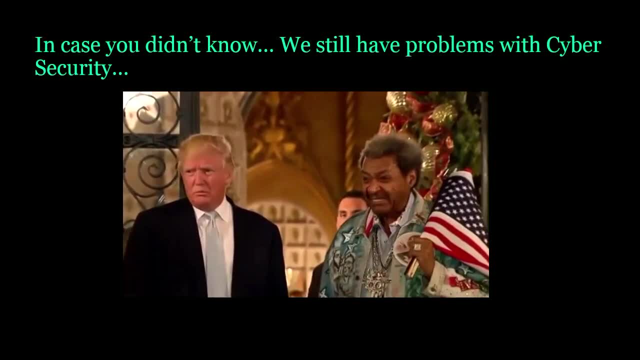 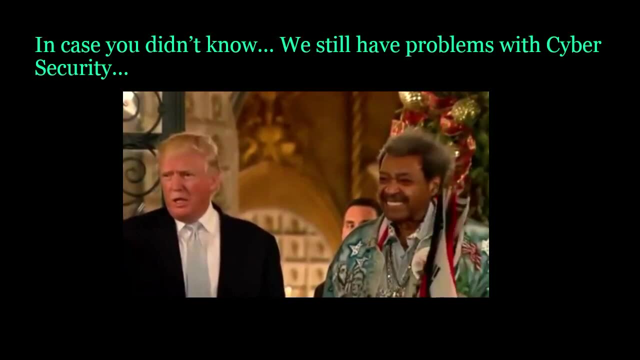 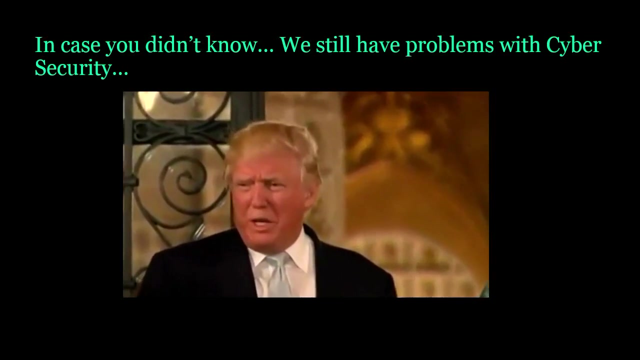 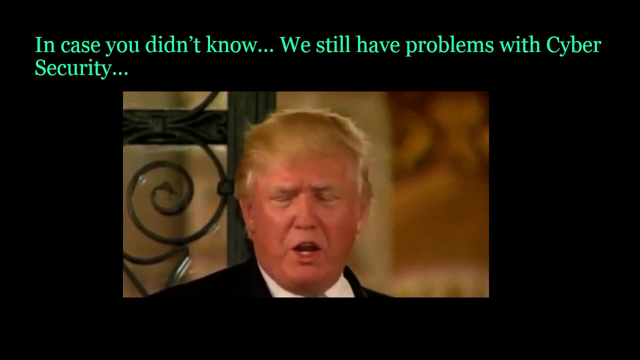 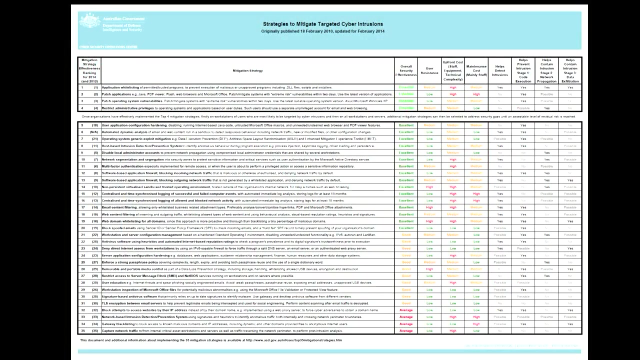 development, And so they have some pretty good stuff there. 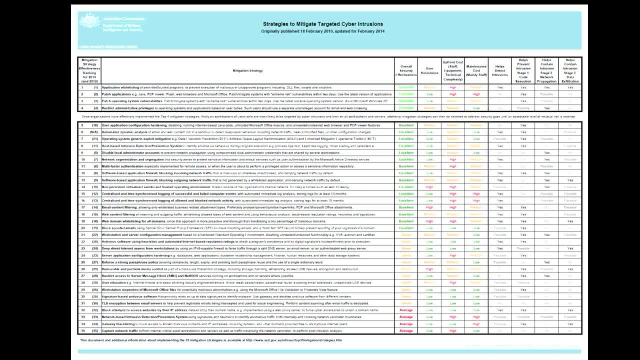 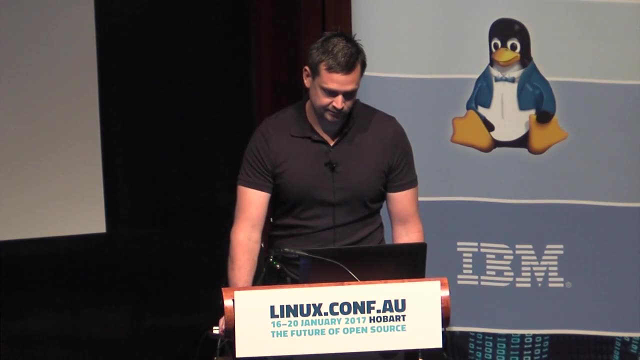 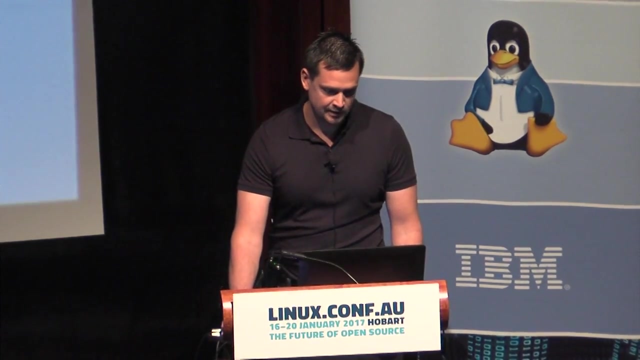 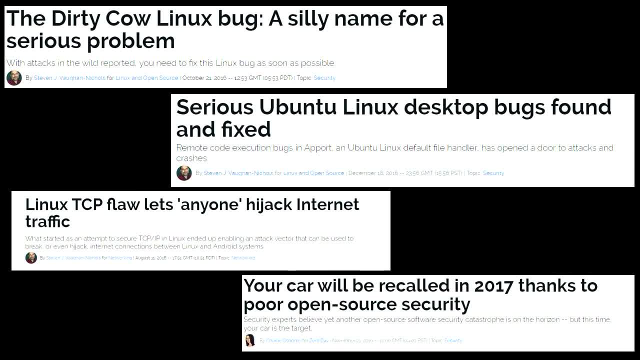 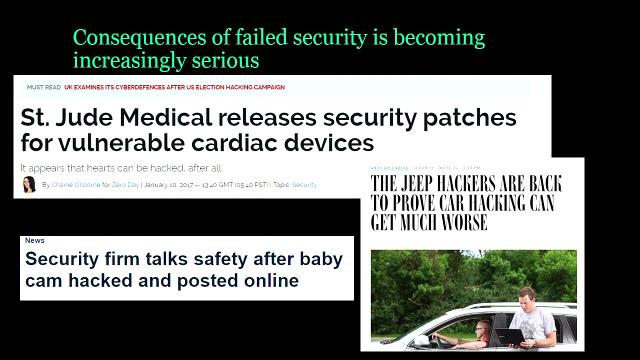 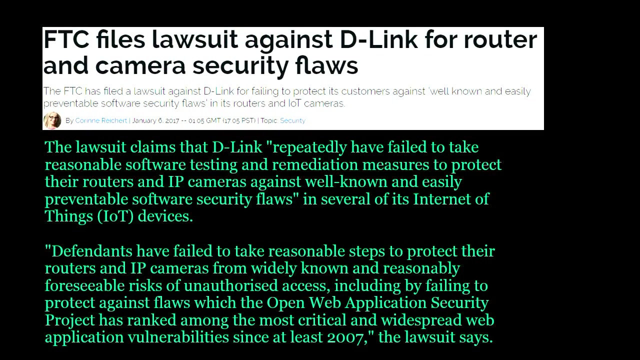 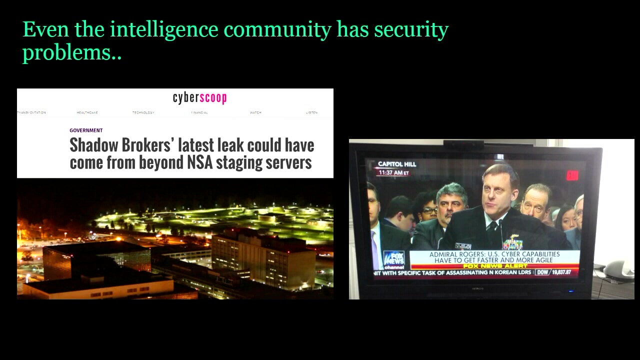 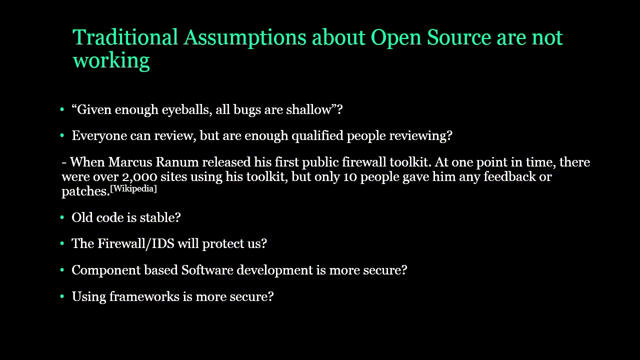 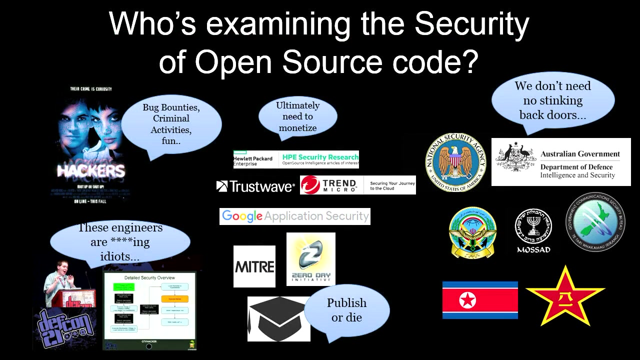 So here's examining the open source security. Well, there is. there are a lot of people looking at it. 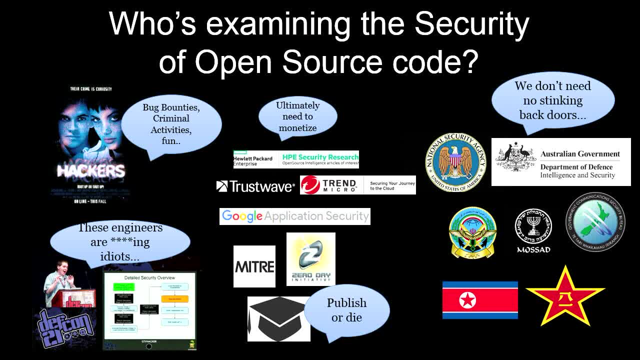 and they have different motivational factors. You know from general kind of hackers that might be motivated by criminal activities. you know development malware or ransomware kind of thing that makes money. There's people that just want to do it for the fun. 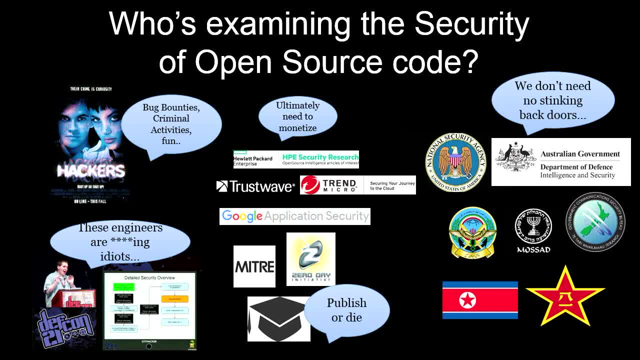 This guy I saw at DEF CON a few years ago when he was talking about a Google product he exploited, called The Engineer, is a Bunch of F'n Idiots, which isn't very nice, but that's a motivational factor too. And of course, you have companies that have sprouted up to want to do research, so they 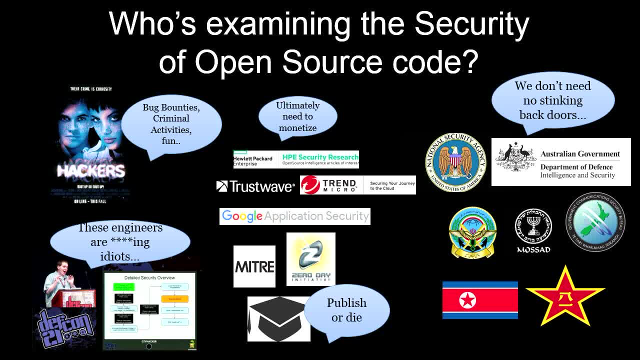 can produce firewalls for you or application layered firewalls for you that can help protect you. Of course, they want to make money. The bug bounty programs want to make money and academia is doing a lot of stuff, but you have a publish or die mentality. 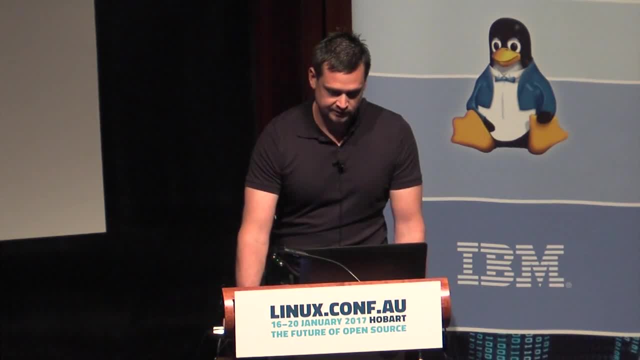 And, of course, your local intelligence agency. they have their motivations as well, and people think about back doors and products and such, but they really don't need them when they can do their own analysis and find issues to exploit. And, like I said, the demand for exploits is really drawing a lot of money, especially. 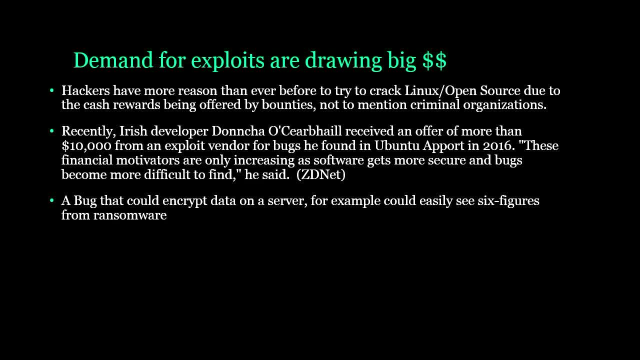 now because the quality code is improving And I think that's a good thing. So the stuff is becoming a lot harder to find. It's becoming more of a specialized industry, if you will. And just recently this Irish developer who found a bug in a port in Ubuntu he said he. 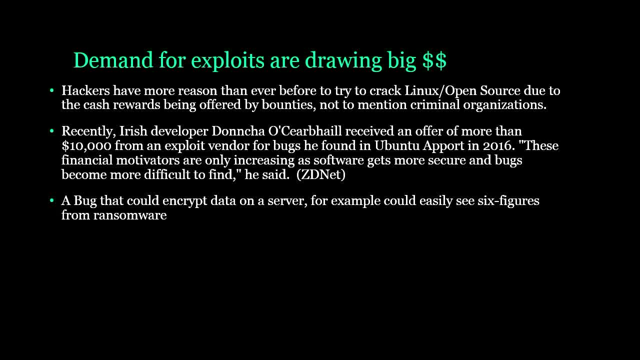 was offered $10,000 for the bug, and if you found something that had to do with encrypting data on a server, surely- and you had a criminal mind to you- you could make certainly hundreds of thousands of dollars on ransomware. 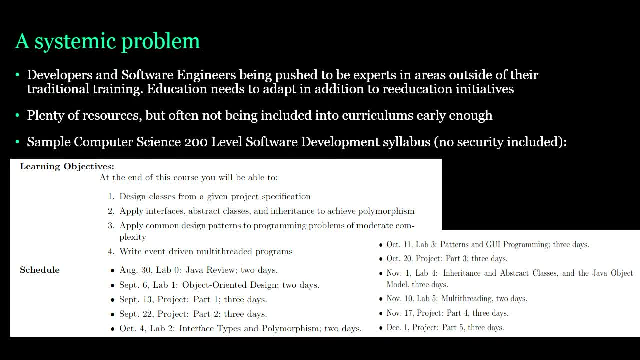 And it's really a systemic problem. It starts really in the typical model that people get into this field. They go to school and study computer science maybe, and they learn how to program as part of that- how to design software. But a lot of times the security aspect is really not embedded into those programs as 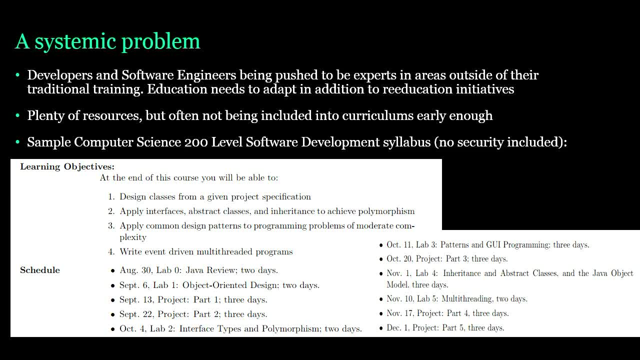 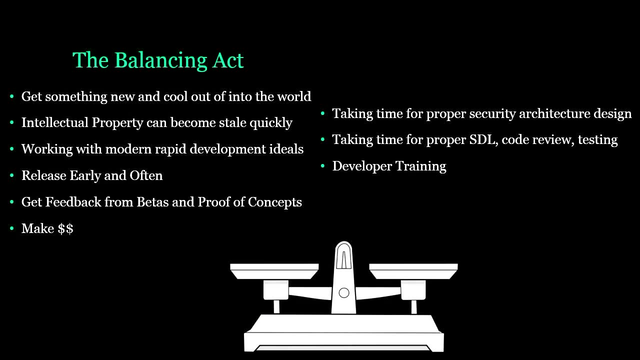 in the syllabus here from the place where I went to school for software engineering, And it's something that really needs to be incorporated really early on into the process. And there's also a balancing act. Of course. there's the idea that intellectual property gets stale quickly, so you need to 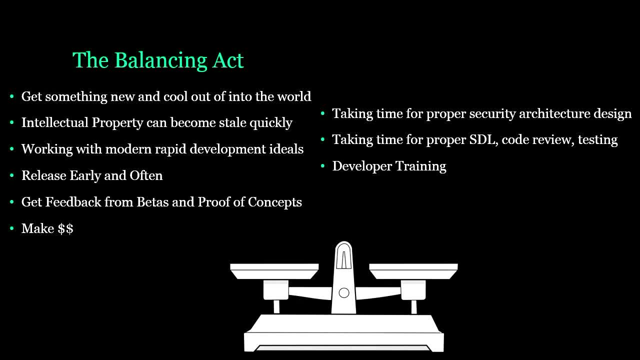 get stuff out the door and you've got modern development ideals of getting rapid prototypes out, that kind of thing. You need to make money maybe. So you know. and then you've got to balance that against taking the time for a secure architecture because, as you know, problems that get into the code that aren't fixed early. 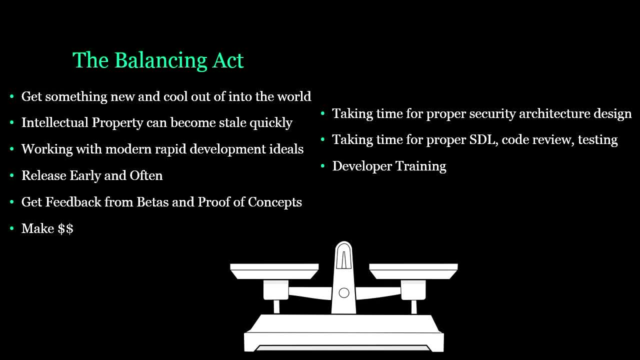 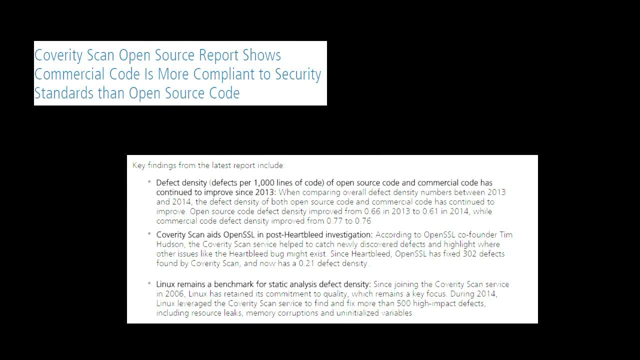 on end up costing more to fix later, Okay, And then taking the time for developer training as well, like I said. So you know this report was put out by Coverity a few years ago. They have a service where they do static code analysis. 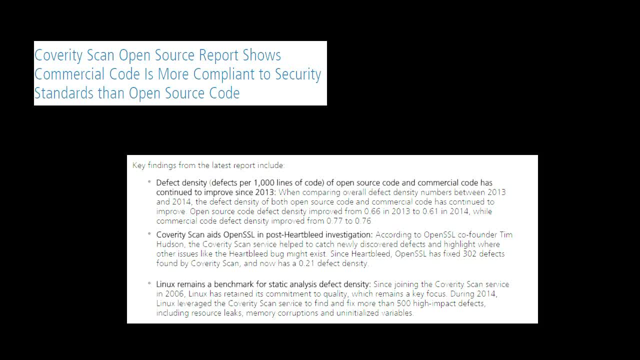 It's free for open source projects and I'll show you that a little bit later here. So in their research they showed that post-source code tends to be more compliant. but that is improving And in fact it's not. 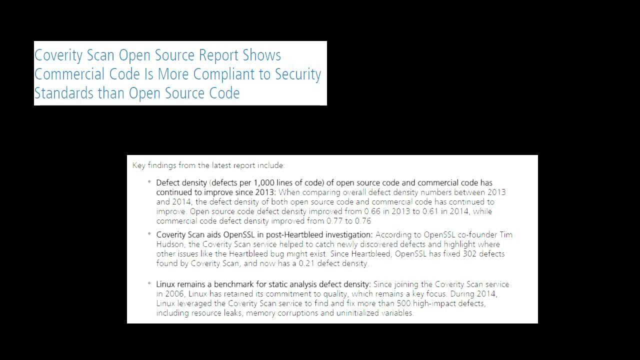 Okay, The Linux kernel itself and quite a few other projects- now I think they said over 5,000, are using their service. Not that that's a panacea- it's not going to find architectural flaws- but it's certainly a good place to start. 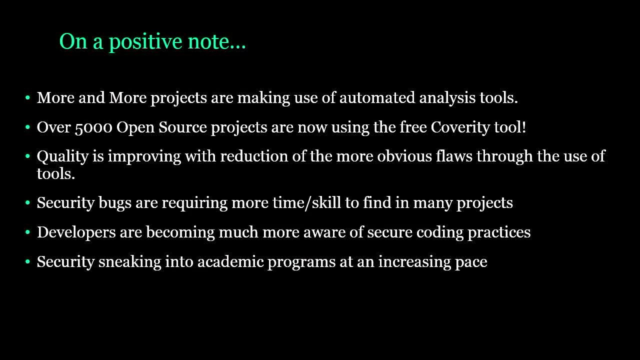 So, on a positive note, like I said, more and more people are making use of automated tools: 5,000 open source projects using Coverity. The quality is improving with the reduction of these obvious flaws that are really easy to catch for static code analysis. 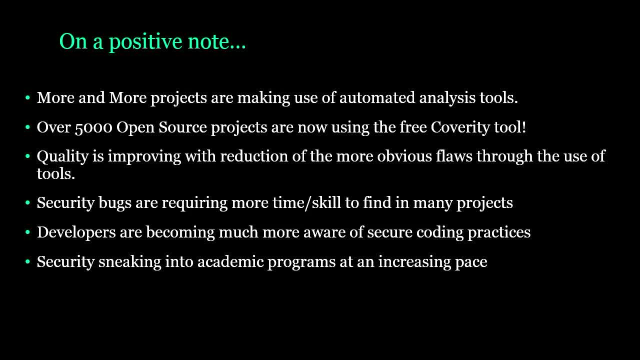 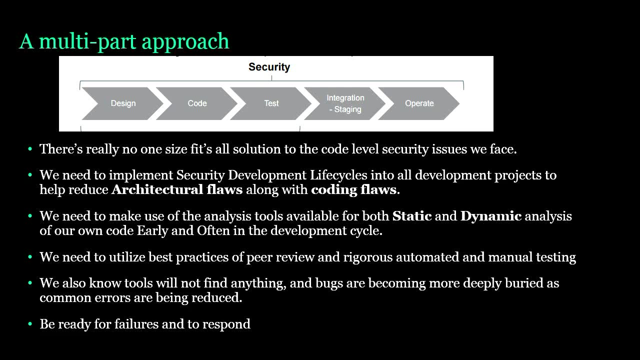 And it's requiring more time and skill. And in academic programs they are starting to sneak some security classes. a lot of times it's electives, but they're moving into that. So, yeah, there's a multi-part approach to this. that's kind of wrapping security around. 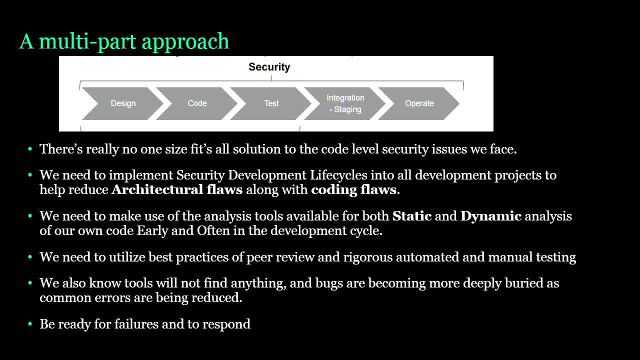 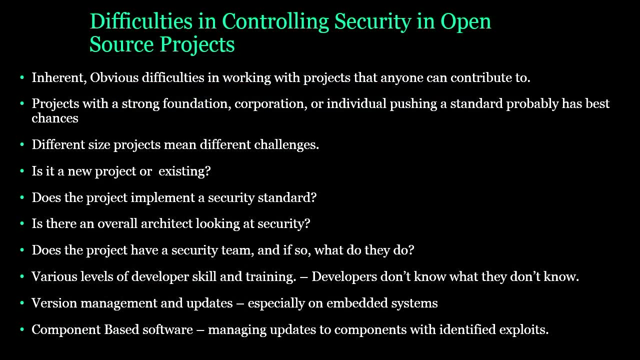 the whole process And it's not a one-size-fits-all solution and we need to think about it when we're designing the code, when they're implementing it and when it's in the operation and support stage. So, of course, in open source projects they have their own difficulties. that are kind. 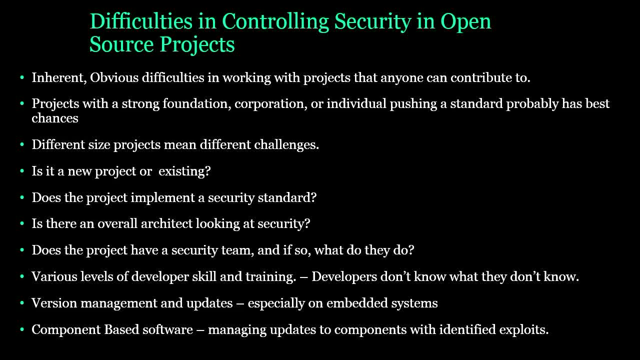 of unique and obvious. I suppose when you're trying to implement some sort of standard- Especially if the project's been around for a while and it's not controlled necessarily by a corporation or something like that- It's getting enough people together and putting out some standards. 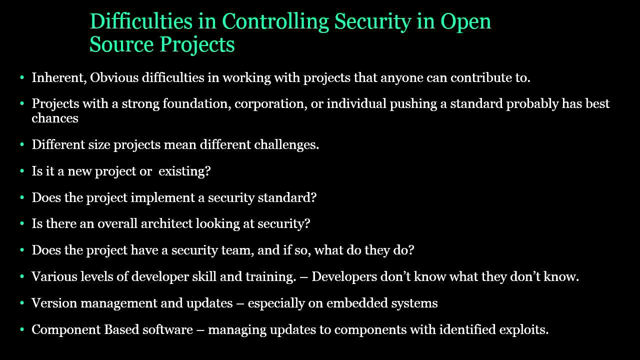 And also convincing developers, So that's a good point. It's good for developers to participate in peer review and to utilize the tools that they can use, And also, of course, you have various levels of developers that are devoting their time. 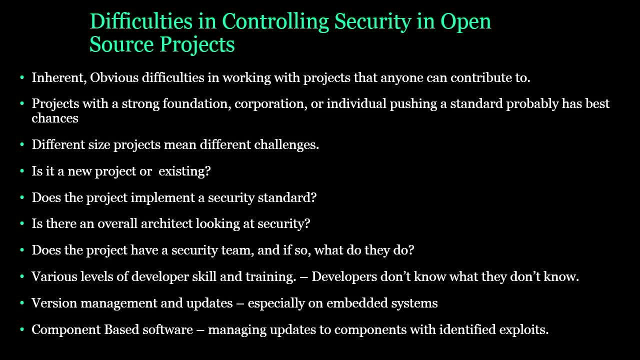 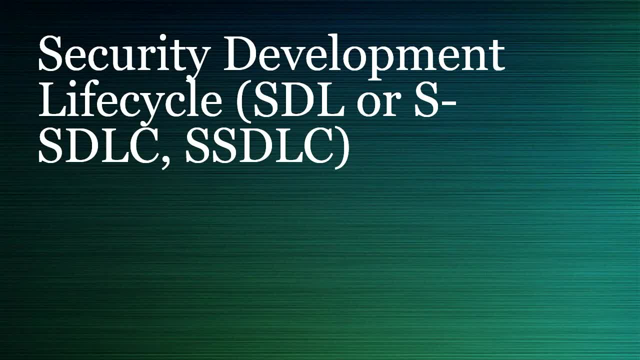 to the project, and some of them may be better than others. So a little bit about the security development life cycle. It's been abbreviated SDL or SDLC, whatever you want to call it. So if you're a project of one or of a thousand, there are certain different challenges of 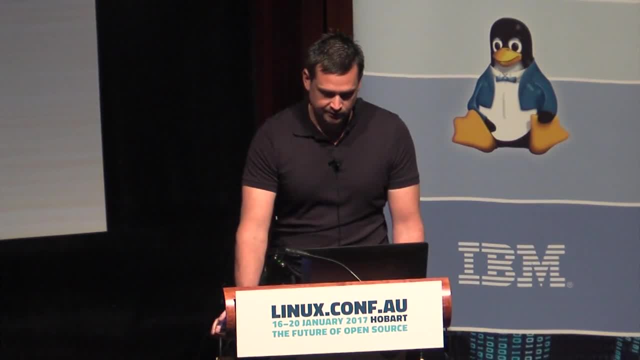 course, in implementing this, But not to mention if it's a company or community, But no matter what the size. I think you could probably take some ideas away from this and apply it to what you're working on, whether it be at work or a personal project or a community. 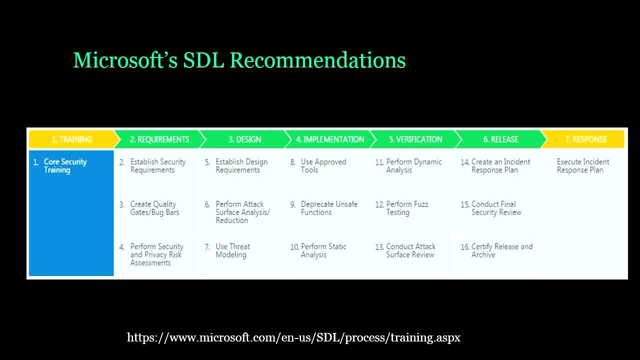 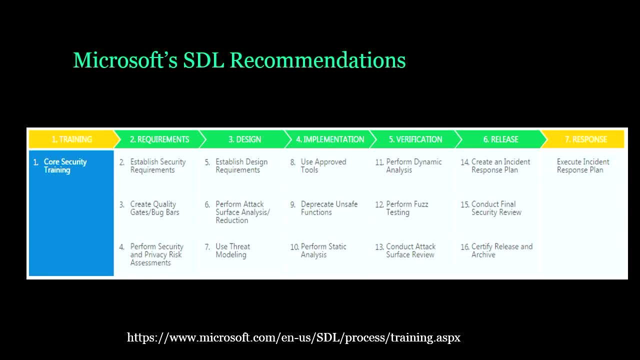 And so they came up with this. It's a bit of a kind of a waterfall model. It can be adapted a bit to Agile frameworks, as I'll show you in the next slide, But essentially you take in the major process areas of development and adding security to. 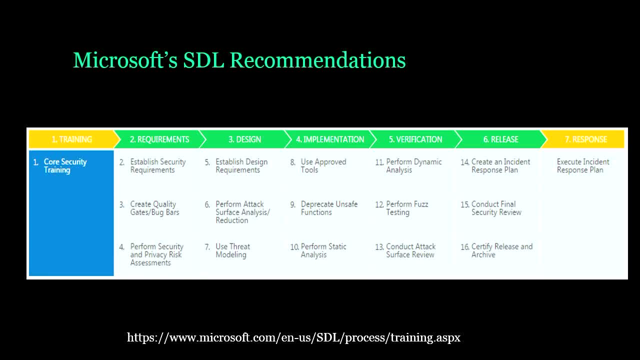 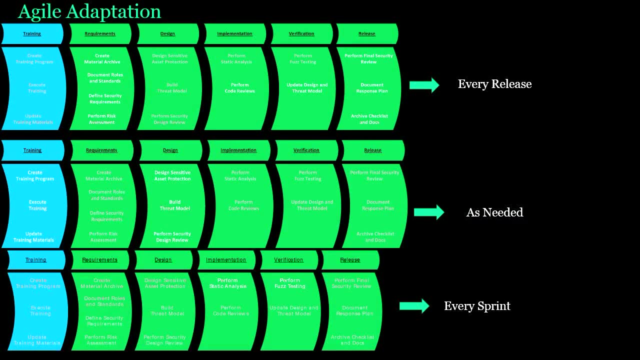 each one of those, And I'll talk about each one of these in more detail in coming slides. But, like I said for Agile, obviously you can split this up as needed. so if you're, for instance, working on the sprint, 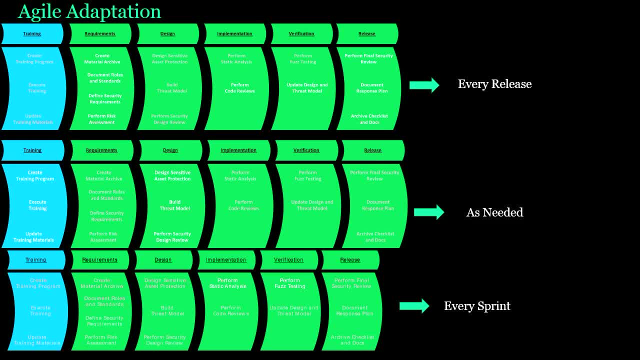 You might go with MTS, not need to do a full requirements phase again, so you can adjust it as you see fit, but pick and choose the major processes out of it that make sense to do- Another thing to look at too. 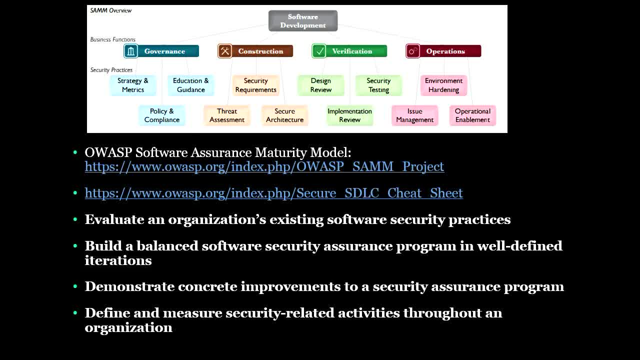 is the Open Web Application Security Project's assurance maturity model. They have a document there that a lot of companies have contributed to and community people and it's more of a higher-level document. if you're trying to implement something for your company, It's not so much technical. 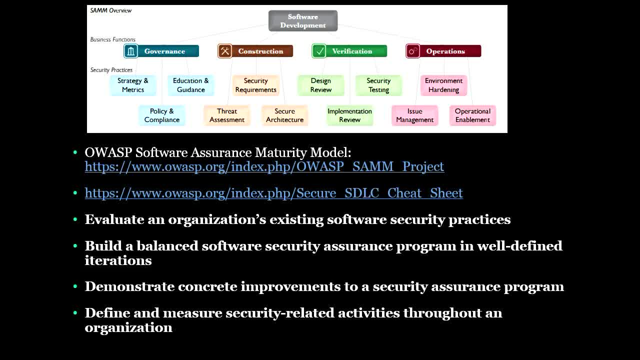 but it's kind of very similar to the Microsoft model, but a lot of the Microsoft stuff talks specifically about their development environments and their tool chains and stuff, and this is a little bit more generic. Okay, so the number one thing and the first thing. 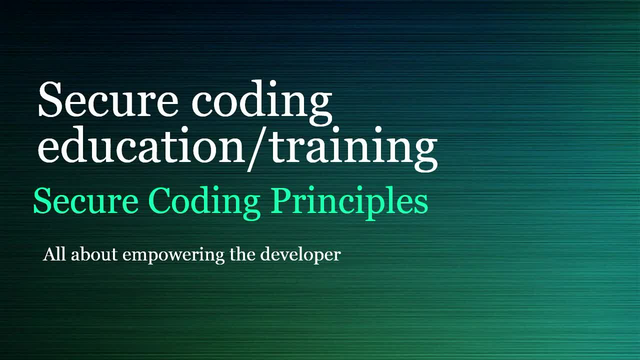 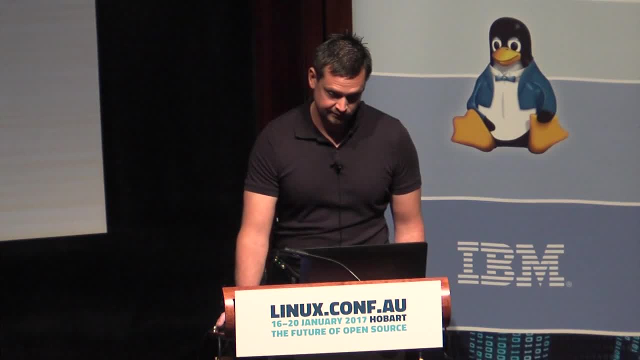 in this lifecycle, of course, is education, training, and it's all about empowering the developer and taking some personal responsibility for yourself, too, if you're a developer and learning about the new things that you're doing. So there's a big difference between security features. 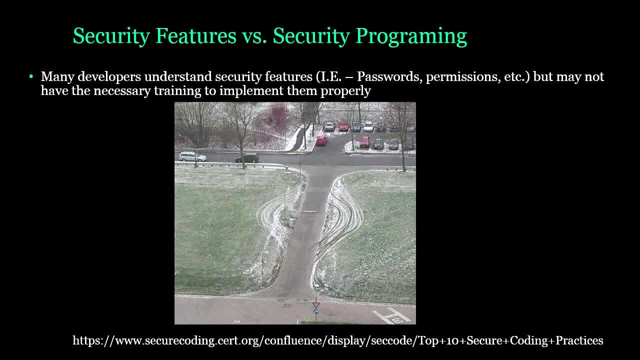 and security programming. A lot of developers understand the need for passwords, things like that. This is a famous picture here. I'm not sure where I got it from, but you can see the security feature is the roadblock, but you can just drive around it. 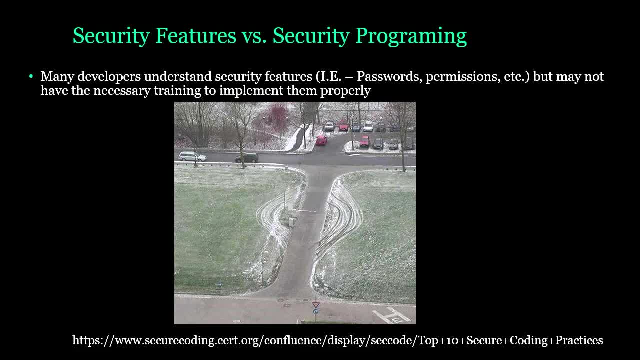 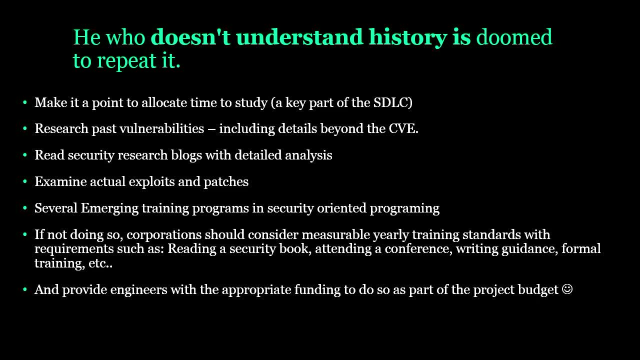 So this is a common problem And, of course, he who doesn't understand history is doomed to repeat it. So you need to make a point to spend some time on the study. You need to research past vulnerabilities that are related to what you're working on. 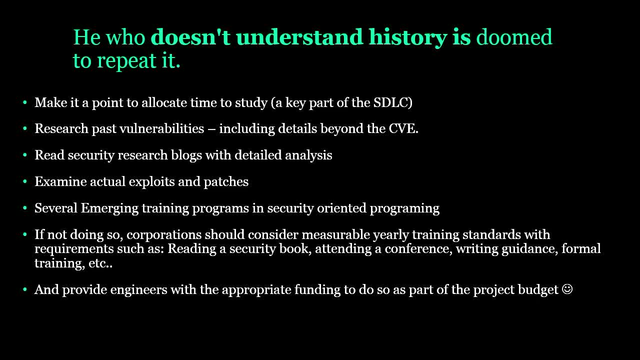 Read security research blogs, especially ones with detail analysis. You can skip past your ZDNet stuff and crap like that and get to some details, And there's also some emergent training programs you can look into as well And, if you're a company, provide your engineers. 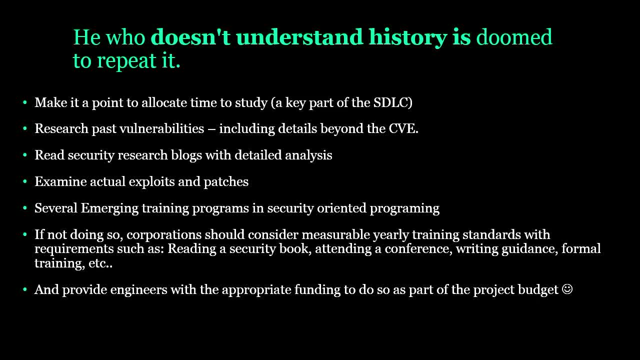 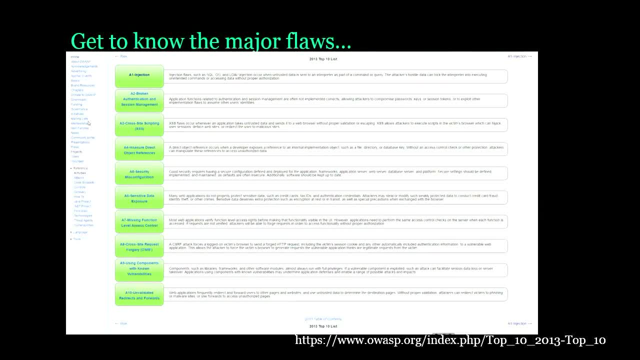 with some training budget too and funding and maybe implement some sort of standardization. that's like you know. you've got to spend a certain amount of hours a year doing training, So get to know the major flaws. These are from the open web application security project. 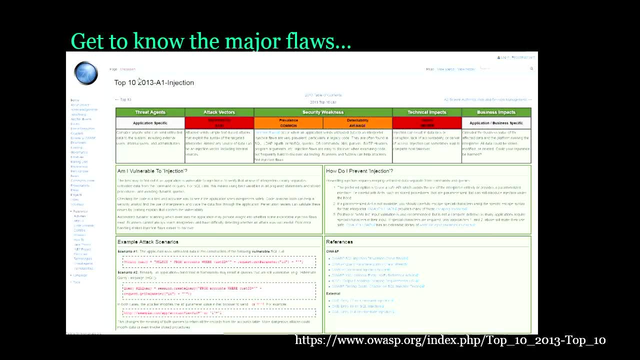 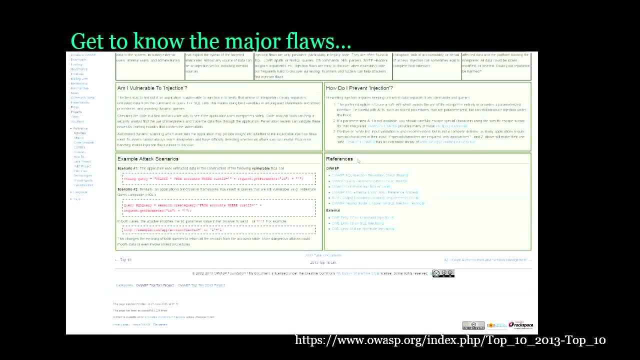 They always have their list. It hasn't been. I think it's getting ready to be updated this year, But each one you can go through and they show you examples of how to recognize it and, of course, how to avoid that issue in your code. 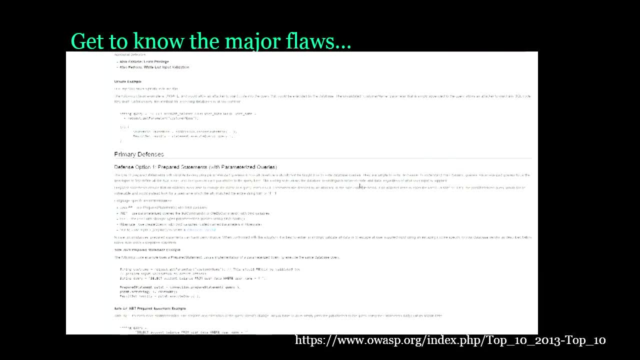 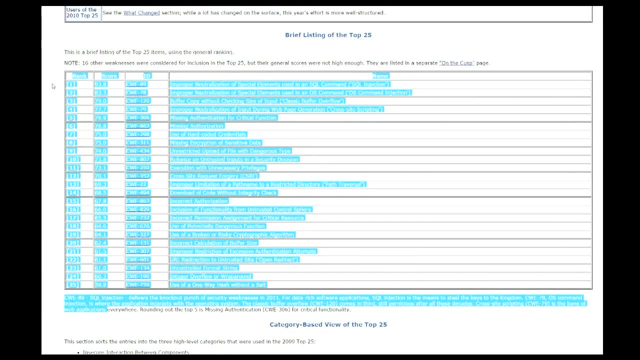 And they Examples might be more generic, so you can always find detailed specifics for a particular language too. Another good place to look is MITRE's CWE, the Common Weakness Enumeration Database. They have their own list of top 25.. 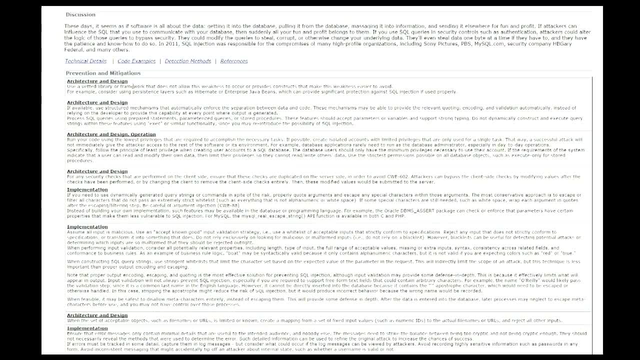 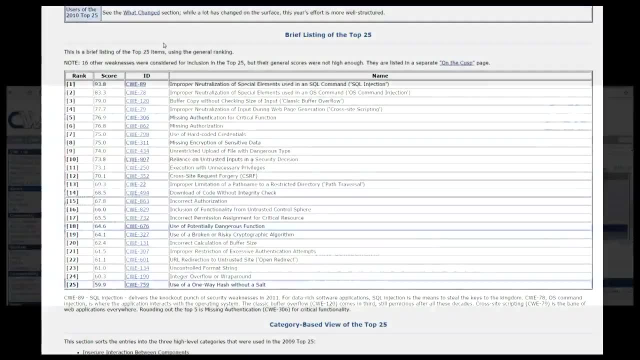 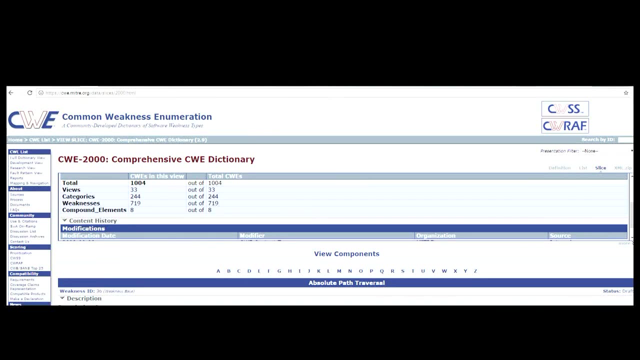 They're highly similar And they also give you some good information on how to avoid those issues. And then so there's over 1,000 weaknesses that have been identified in this database. I'd like to maybe take a little time. when you are doing your thinking about the project. 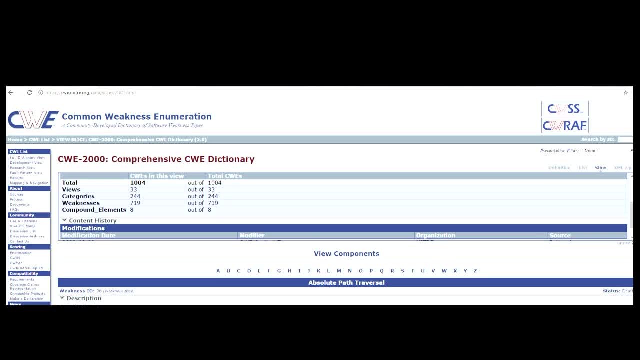 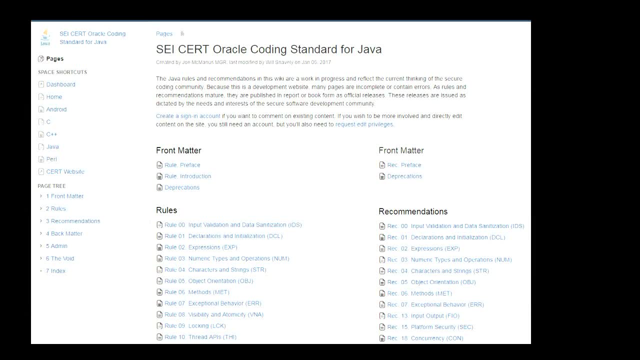 to look for some that have been shown up in other similar projects so you can kind of understand what you might be up against and some ways to go against it. And another thing to consider is looking at the Carnegie Mellon. Mellon has some secure coding standard documents. 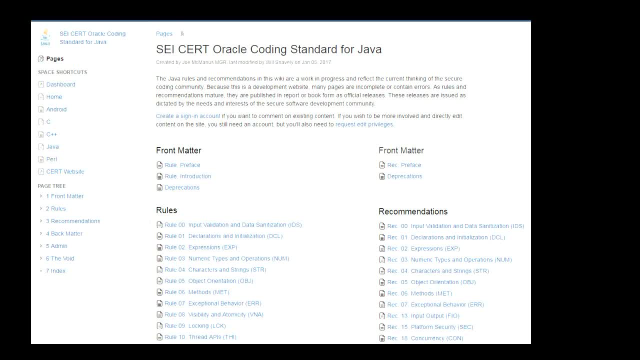 that also give you some tips on how to, well for one, like stylistic things, but also how to, you know, avoid some of the common flaws as well. This guy, David Wheeler, has got a free book. 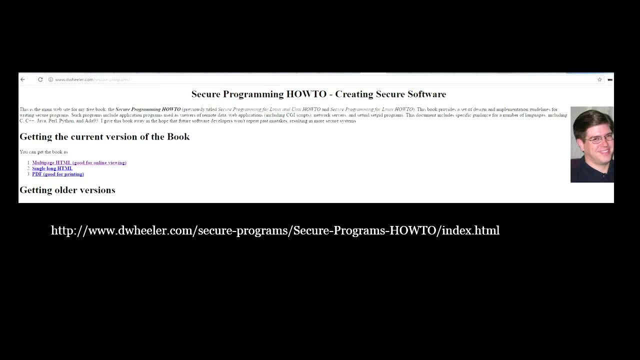 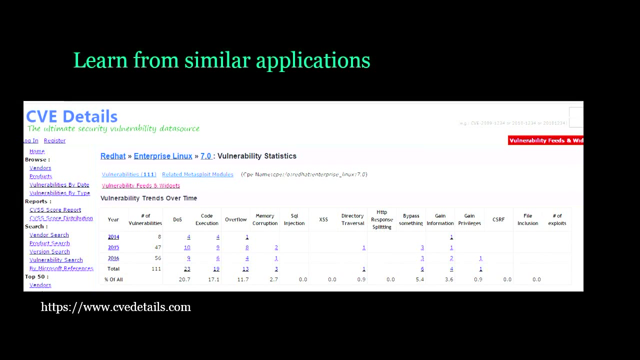 He created the Static Code Analysis Tool, FlawFinder, And it's a free web book. It's worth looking at. It's kind of focused on open and open source and Linux in particular. Like I said, this is another site, the CVE details. 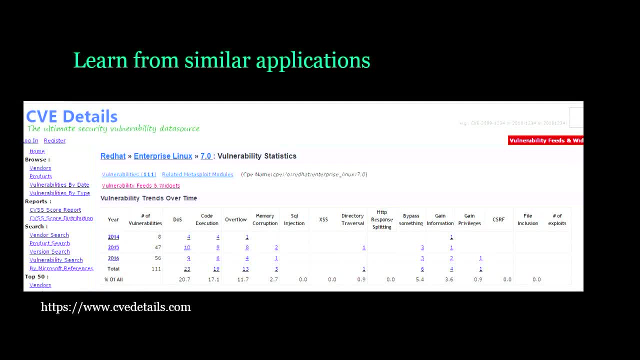 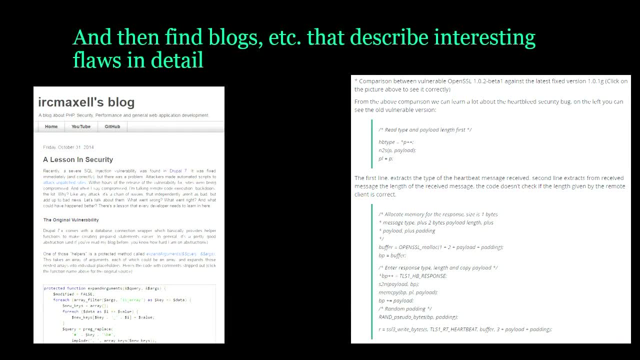 You can look at similar products And they have it broken down by the type of vulnerability and do a little research on how they might be related to what the product you're working on, And then, of course, find a blog that really gets into the details. 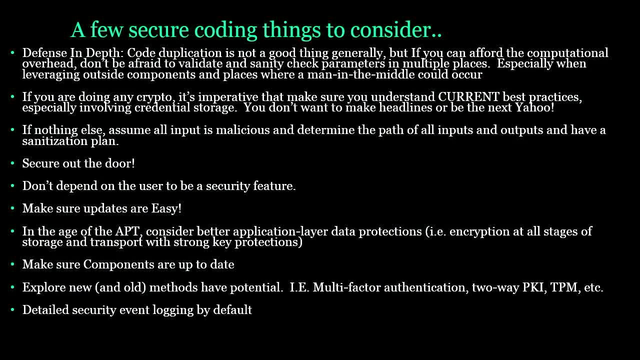 A couple of secure coding things to consider. Defense in depth is something thrown around a lot, especially in the DOD, But people try to avoid doing code duplication. But in some instances, if you can afford the performance penalty, you're getting some data back from another outside framework. 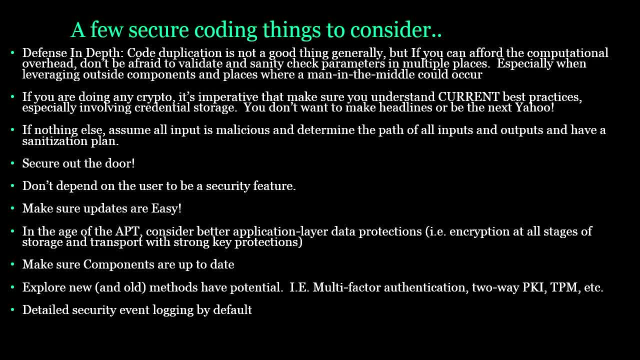 that's supposed to sanitize the code. Maybe, yeah, look at it again. Do another standard thing. Yeah, Yeah, Yeah, Maybe check on it before you do something with it. that's dangerous. Don't depend on the user, of course. 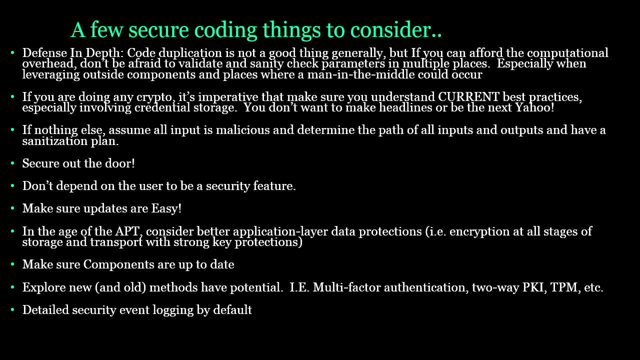 It'd be a security feature. You make your updates easy. Consider new ways of protecting data in this age of APT, like encryption in all stages, from network transport to storage, with strong key protections, multi-factor authentication And, of course, detailed security event logging. 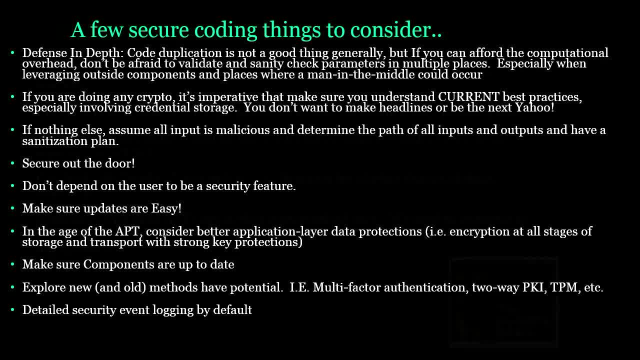 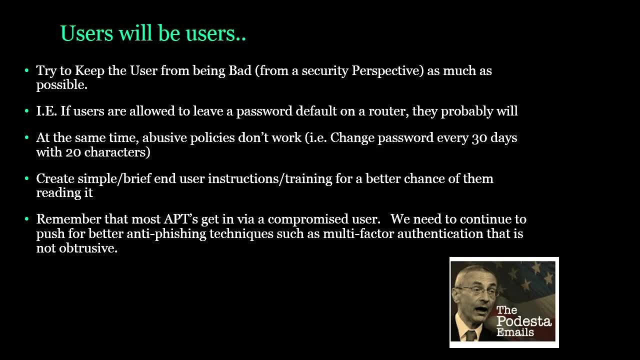 So when something goes wrong, people are used to it. They're using your stuff and kind of figure out maybe what happened, And users will be users, Of course. keep that in mind, You know, if they're allowed to leave things in insecure state. 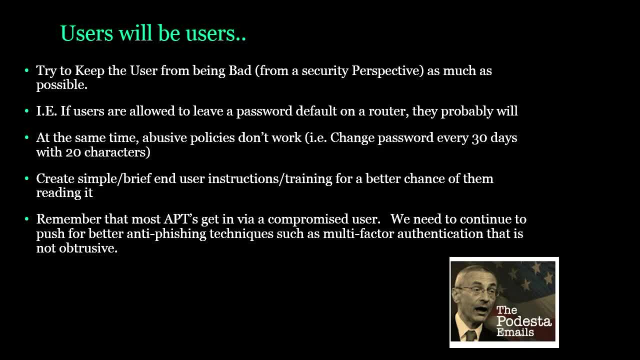 they probably will. So, if you can think of ways to you know, force them to randomly generate your password for some sort of IoT device, for instance. But then again, don't be too abusive, because if they have to change their password 30 days, every 30 days. 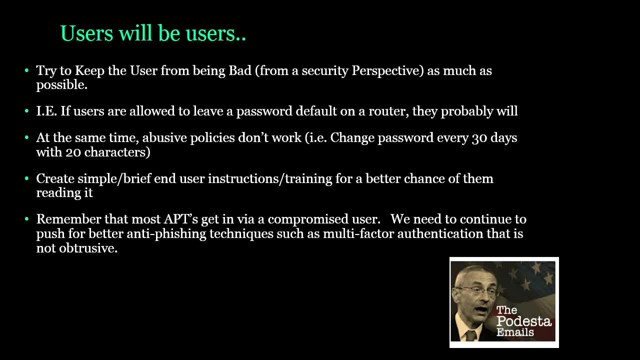 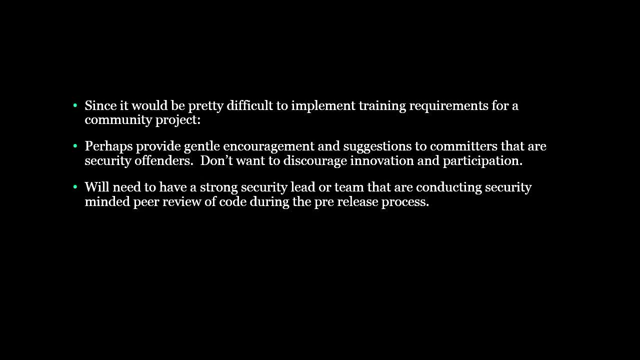 and it's 20 characters long. they will make bad passwords and write them down and stuff. Yeah, And you know, I think that's something that's important And, like I said, it's difficult to do this in a community project. 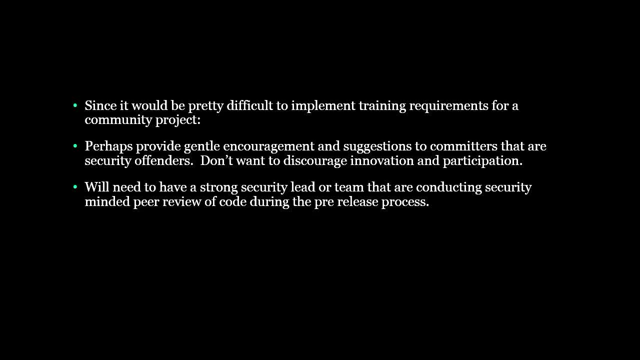 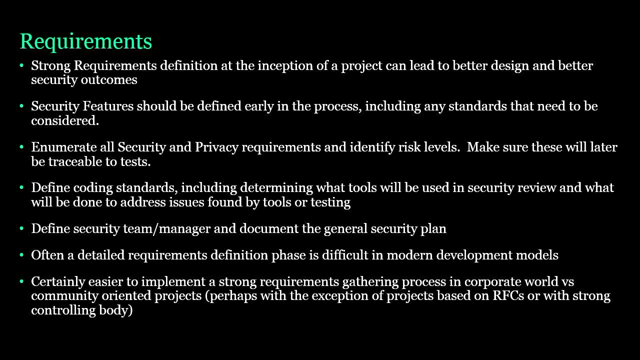 but it provides gentle encouragement if you're doing code peer reviews and you see somebody making mistakes. So requirements: nobody likes really this phase. I think developers might not, But it's a good time to tease out some of the security features that are going to be implemented. 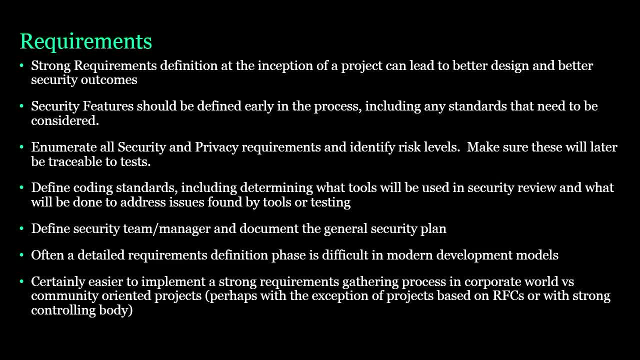 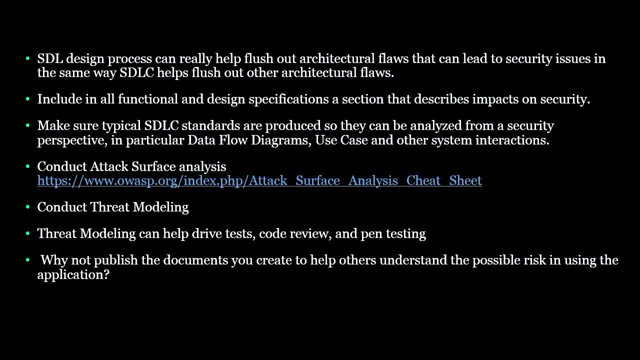 And it's going to be a way to enumerate some of the risks early on in the project And in the design phase- probably one of the most important parts- to avoid architectural flaws you're going to want to try to flush out for your standard software design documents. 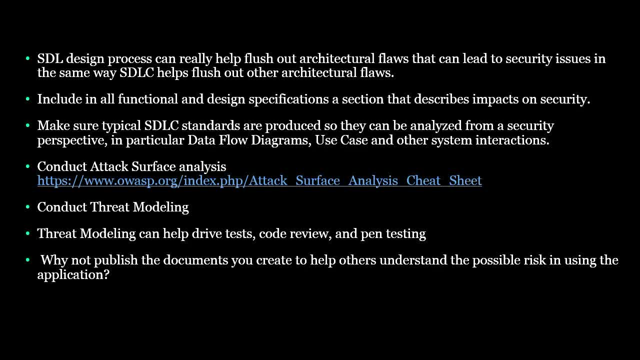 like your data flow diagrams, user interaction diagrams, and kind of convert those into attack surface analysis and threat models. And I say, why not publish these documents at the end of the process too? because that way you know whoever's going to be using your system in the end. 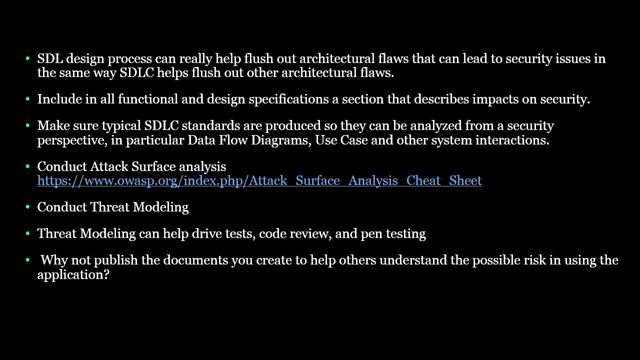 your application in the end can think of their own ways to work around some of the some of the security concerns that come up in your threats. that add a multi-layer approach. Attack service analysis is simply looking at all the paths that data is coming in and out of the system. 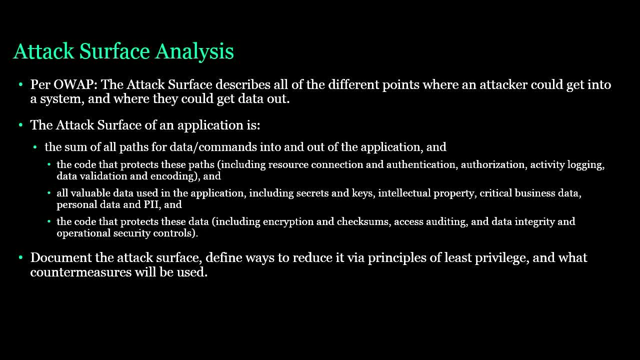 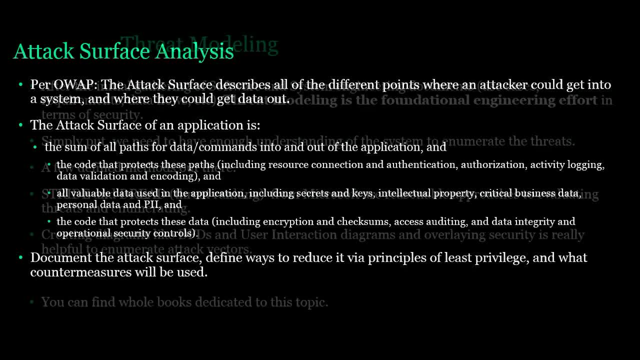 and recording essentially what you're going to do about it. This way, when you go back into when you're testing your code, you can go back and look at this and make sure everything that you initially thought of is going to be covered in your test cases. 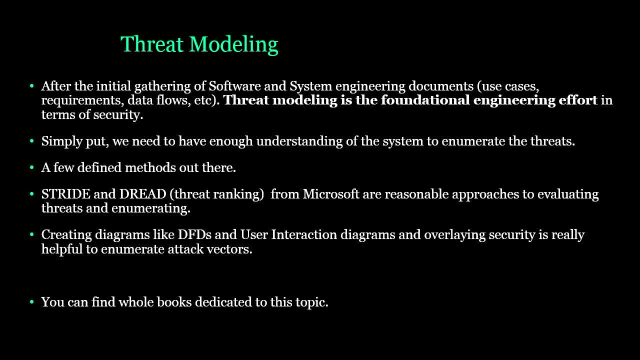 Threat model is probably the most important. You can read a whole And it's essentially taking your data flows and inserting trust boundaries into them and also ranking the type of threats that you're going to see in terms of their likelihood and what they're going to do if they, how much damage they might do and kind. 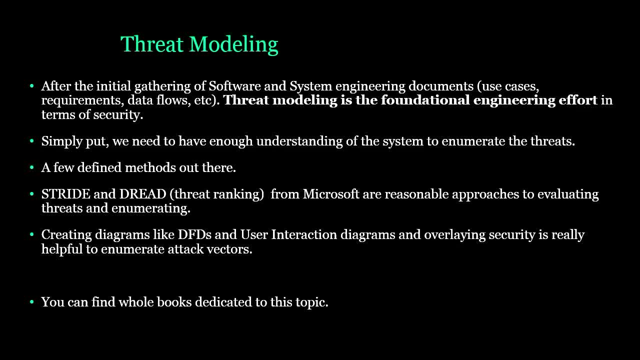 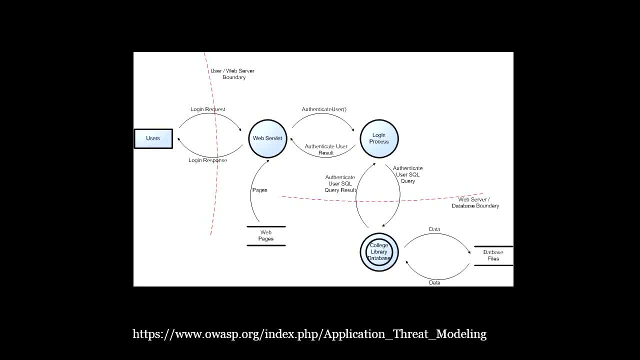 of stack that in your- I don't know your- queue of how important it is to address. This is an example threat model where you took a DFD and added it to your data. This is an example threat model where you took a DFD and added it to your data. 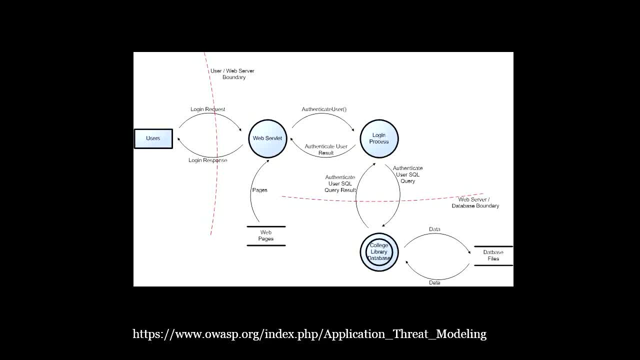 This is an example threat model where you took a DFD and added it to your data. This is an example threat model where you took a DFD and added those dotted red lines which are the threat, excuse me, the trust boundaries and, essentially, where data is coming in and out from an untrusted source. 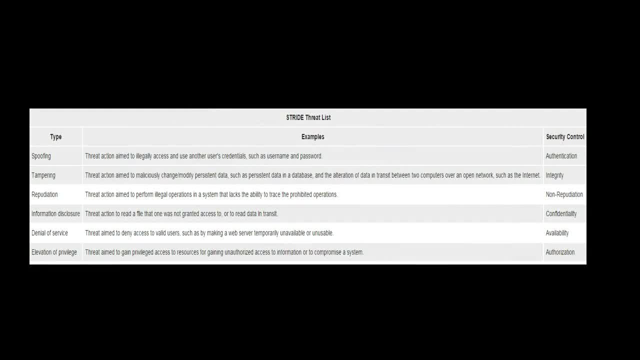 Stryd is a way to kind of document those types of threats and they're based on spoofing, tampering, repute, non-repudiation, information disclosure, denial of service and elevation of privilege. So you can go through and create a document that has these different kinds. 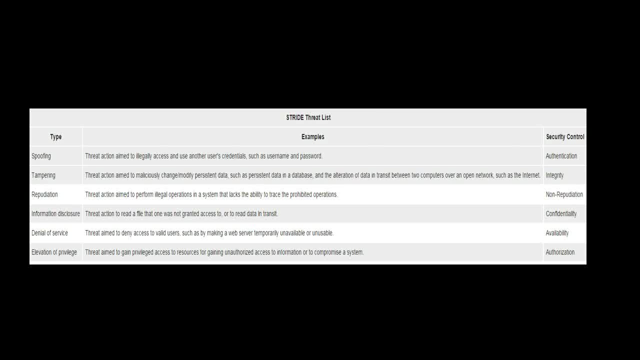 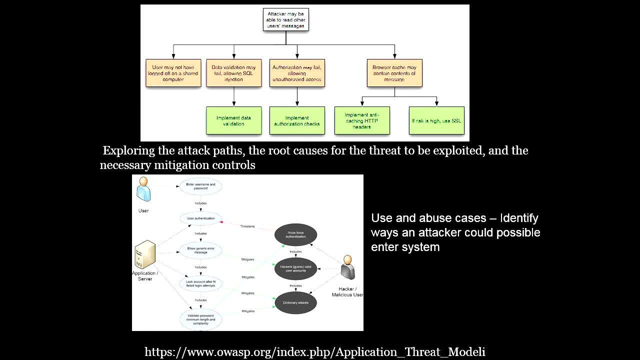 different things and then conversely what you're going to do to mitigate those in terms of security control. and then it can be helpful to diagram, like shown here. you have root path analysis in the top diagram and ways that you're going to mitigate it there on the bottom, the green blocks. 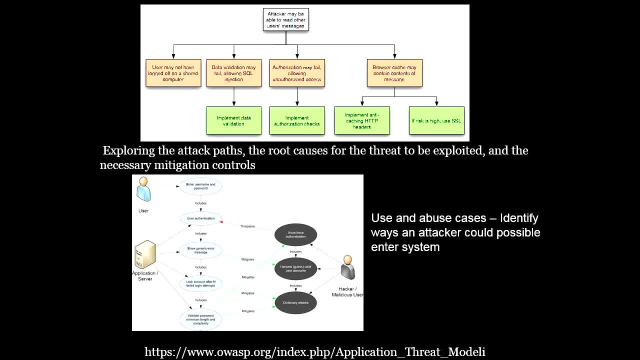 and use and abuse cases. take the use cases that are diagrammed and also and add a hacker- you know a malicious user and uh, and show points where he's going to possibly attack. these are places that you're going to want to focus on more when you're actually implementing the code. 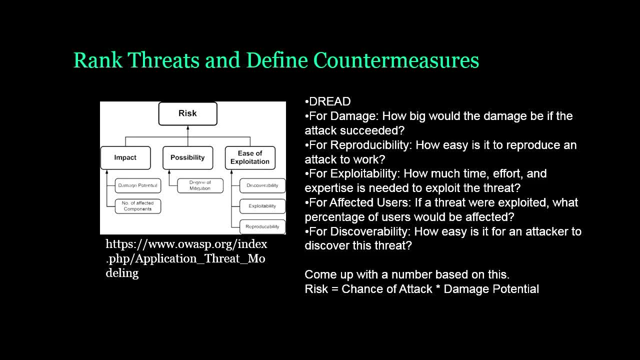 and so dread is a way to rank those threats. if you have the time to do that, it's a way to focus your your attention to the most serious things when you're doing your code reviews and you know, even a well-thought-out design can fail. one of the things i threw in my headlines 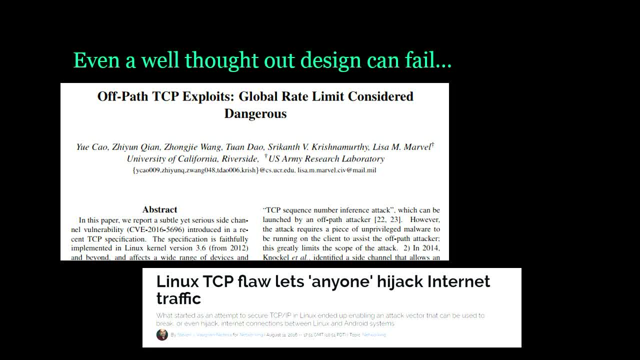 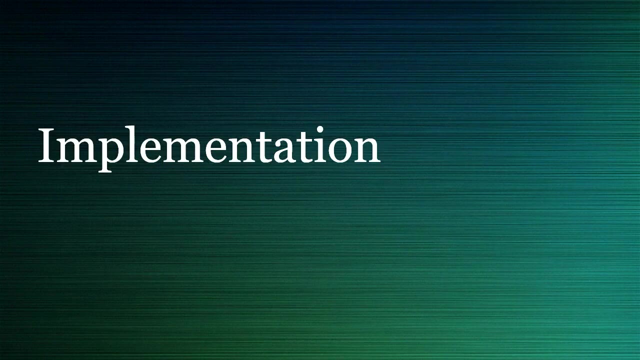 earlier was that tcp flaw. that was actually based on a fairly well-vetted rfc that that linux implemented faithfully, but some researchers spent a lot of time peddling with it and and realized that it could be. it could be broken and to major consequences. supplementation phase is where you are going to implement the project, of course, and 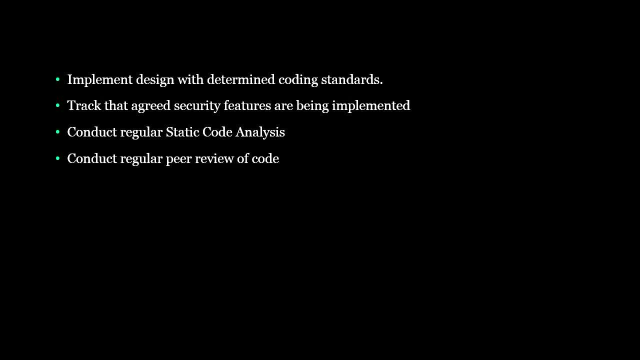 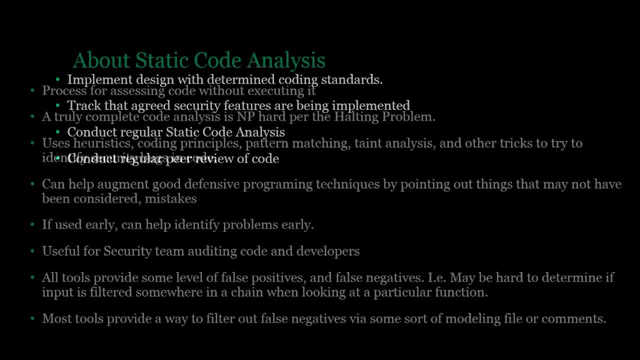 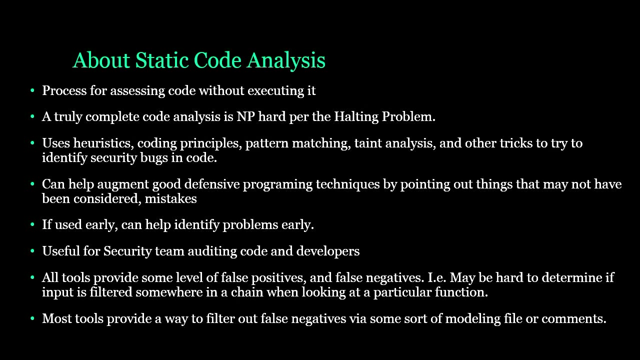 implement with the coding standards you decided on, and track the agreed security features, make sure they're being done, and also conduct regular static code analysis. and regular peer reviews is probably even more important. the static code analysis is a process of assessing the quality of the code without executing it. it's really if you're a computer. 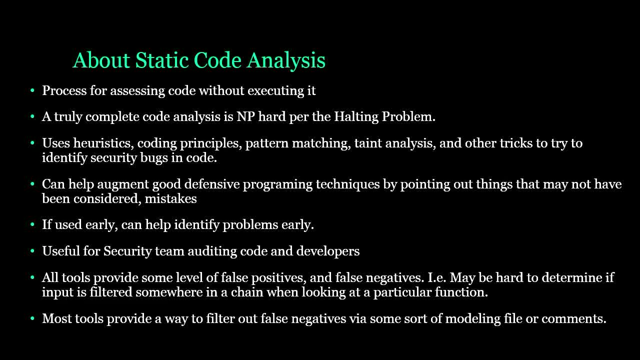 science problem. it's an mp hard problem, so you can't really do it to 100 percent detail. so to get around that, there's a lot of different ways that these tools work, including heuristics, pattern matching, things like that, and the different tools do this slightly differently too, which hopefully 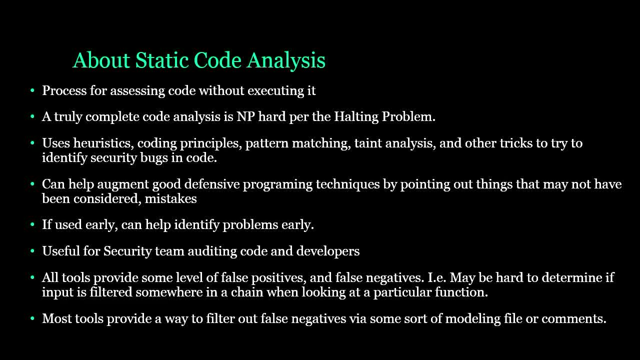 i'll have a second here to show you a couple of ways that they're different. and use it early in a often tie it in with a continuous integration server, if you can, if you're doing that type of development, and then each day you know, whatever the build happens, you get a report back and kind 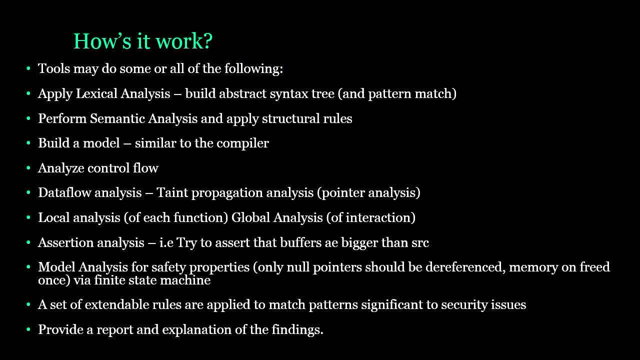 of try to address things as you go along. um, so i don't have time to get into all of this, but they work different ways. like i said, it could be a simple pattern match type of thing to something that builds a, a model based on kind of similar way that the compiler works and then conducts. 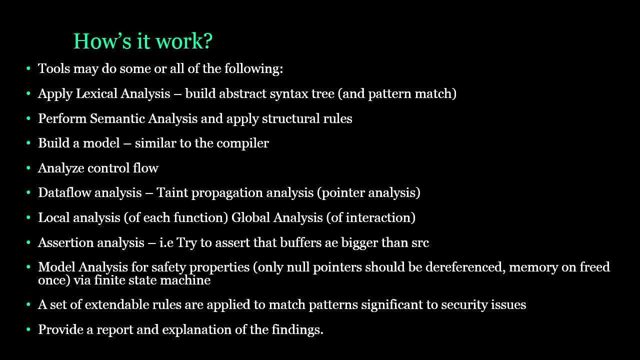 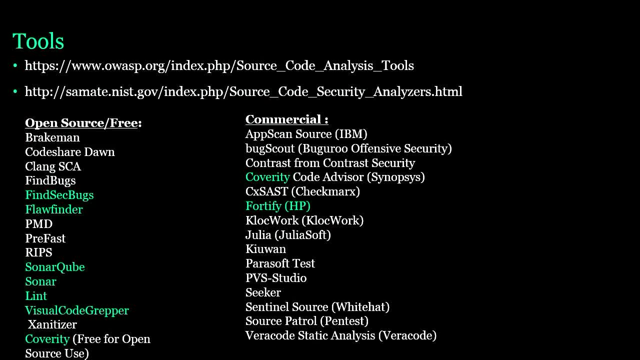 like a data flow and taint analysis to try to figure out where stuff is coming in and out of it and how it's coming in from user input or network input to make sure you're sanitizing the input. here's some, some tools. you can find some list of them out there. i was going to show you. 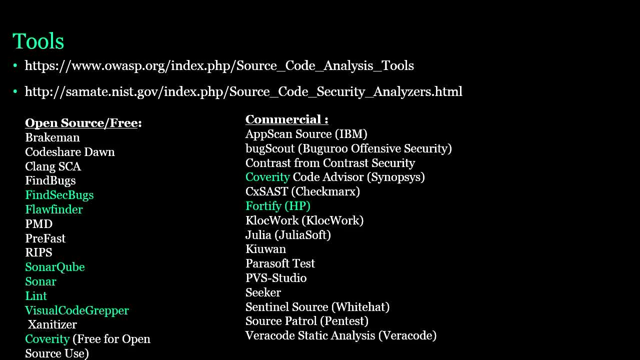 hopefully the coverity might have to not take questions if i do it, but i think it's important to show you a couple tools. the coverity thing is a commercial tool but it's free to use for open source projects. i highly recommend signing up for that. you can also find a lot of projects that. 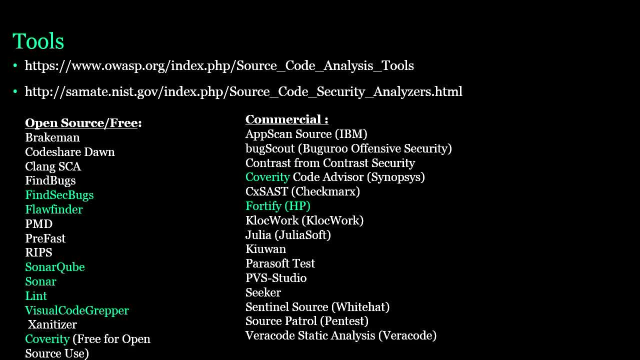 are on their site. if you are a contributing member, you can request access. they probably will not give it to any random person because they don't want security researchers taking advantage of this and, you know, finding flaws and when these people are really just trying to improve their code. besides that, the fortify product i'm going to show you, there's a sonar. 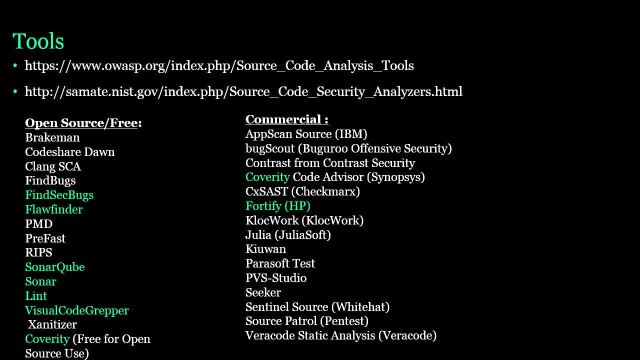 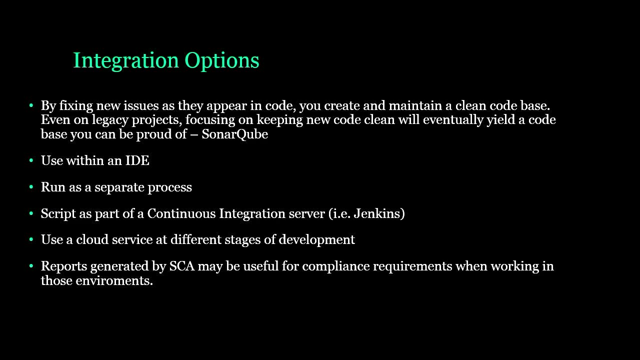 as a also a free end. they also have a commercial product, a visual code grepper and find security java thing. that's could be plugged into eclipse. i like to say you have different integration options, whether it's an iee running as a separate process or continuing integration. there's also 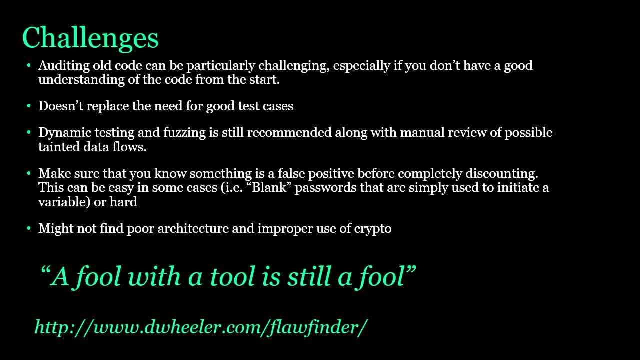 cloud options as well. challenges: if you're auditing old code it's. it's a pain i mean you got, and especially if you didn't help develop the code. it's a really difficult thing to do from start. that's why it's really good to do it when you're talking about new projects and getting it in early. 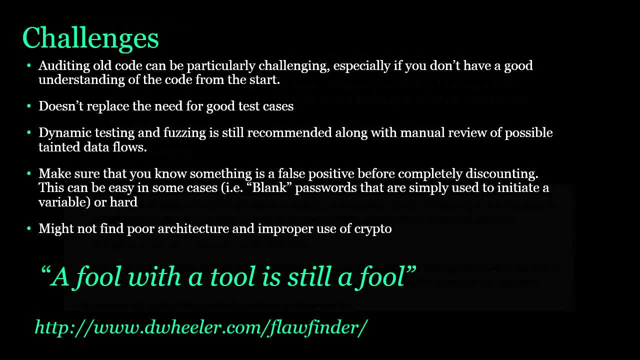 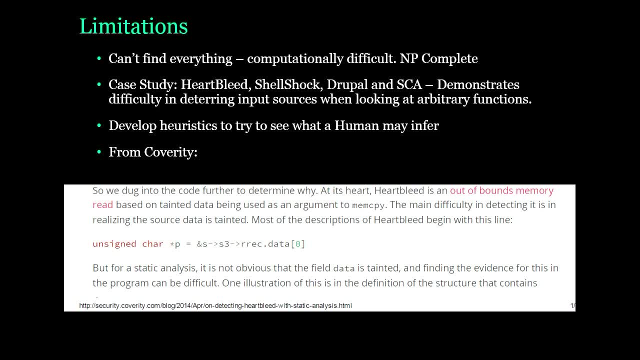 in the process and it's still recommended. do dynamic testing limitations? i can't find anything, everything obviously, just didn't find shell shock. i didn't find, although since then they've improved some of these tools to be able to detect the issue to cause shell shock, which is just better taint analysis. 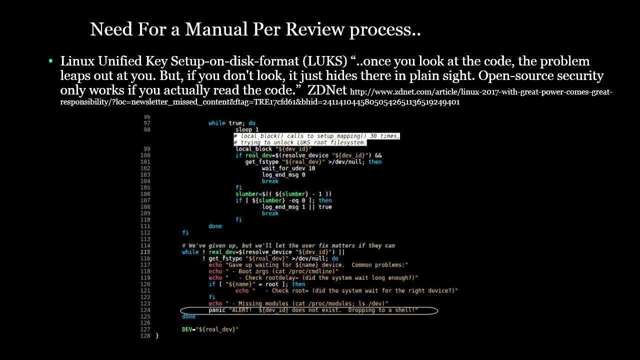 and there's still a need for manual peer review. so you can avoid something like this- which actually wasn't a problem with this key- that this application stuff like one of the setup scripts where it dumps to a shell if you hit the enter key more than 30 times. 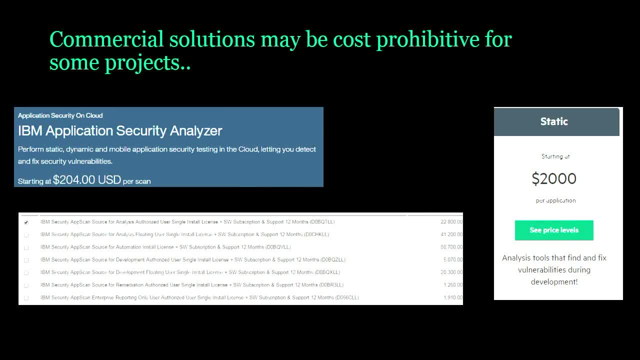 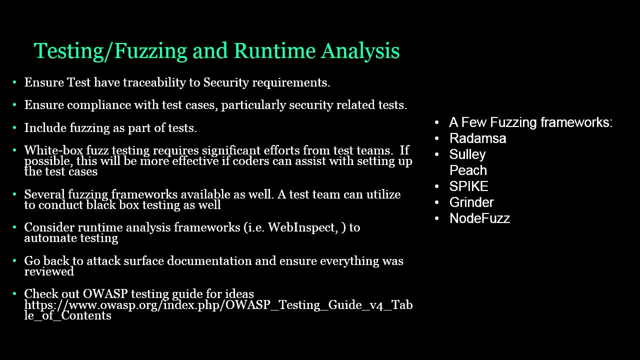 and commercial solutions can be cost prohibitive for open source, of course, too, and verification is important after you, before the project is at the door of the fuzz testing and runtime analysis if possible. if you have a good test team, they're going to utilize these tools. it's really good if a developer can help write fuzz testing and dynamic. 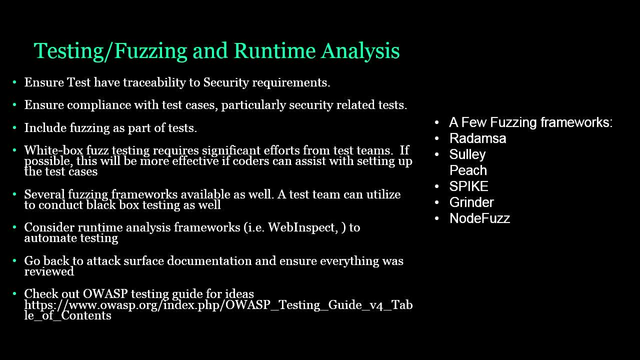 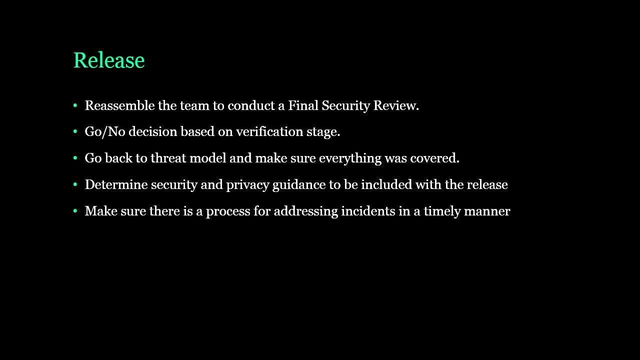 testing because they know the code and they're the best people really to help assist with that process and real quickly. of course, several the final team to conduct the final security review, no go, no go decision and of course, try to to document anything in your in your documentation. 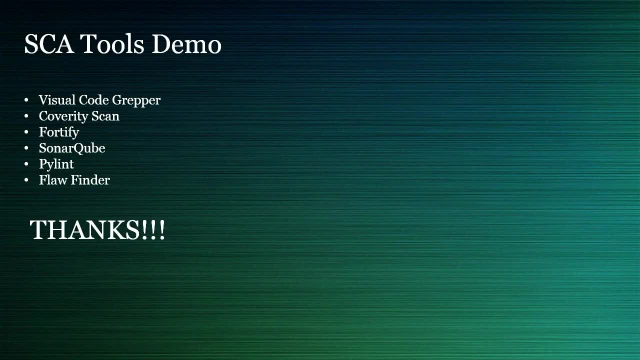 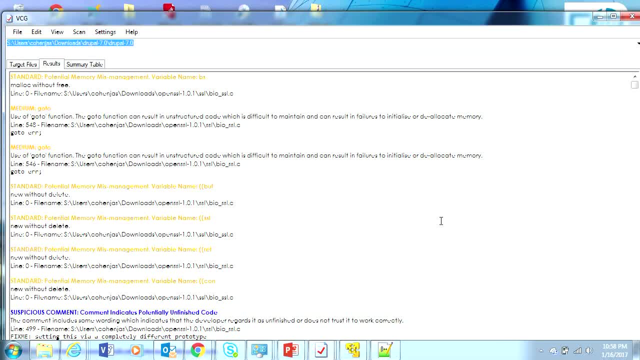 all right, how do i know crap matching for different known kind of bad coding properties, but it doesn't look at the code overall. This is an analysis it did of OpenSSL, a vulnerable version of it, And then it can give you a nice little pie chart. 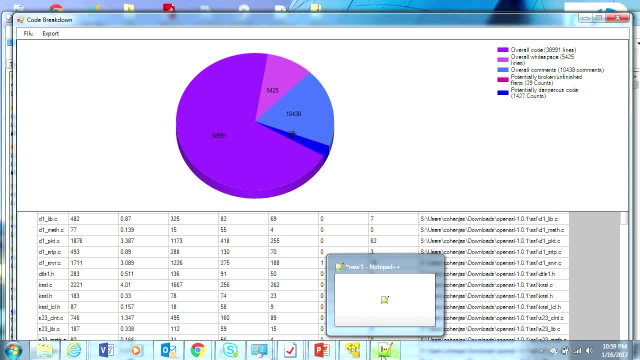 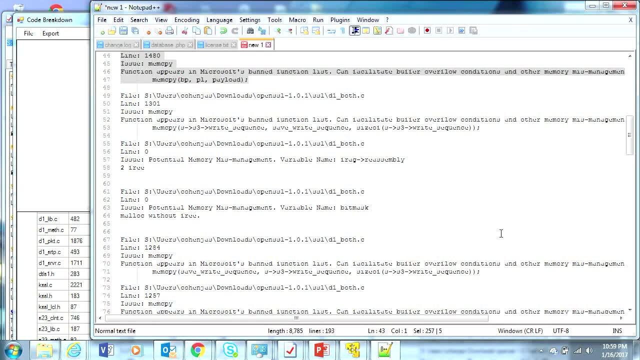 with places to look And then if you pull up a particular file that it analyzed, it'll walk through the different things. Now, like I said, if you're looking at an old project, you're going to get a ton of hits with this. 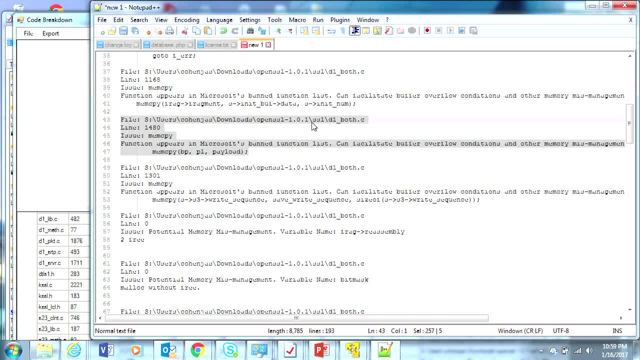 And it's going to be kind of difficult to go through, although the highlighted line there is, in fact, where the Heartbleed vulnerability was. So I suppose if somebody really did this and looked through it, they might have found that and fixed it. 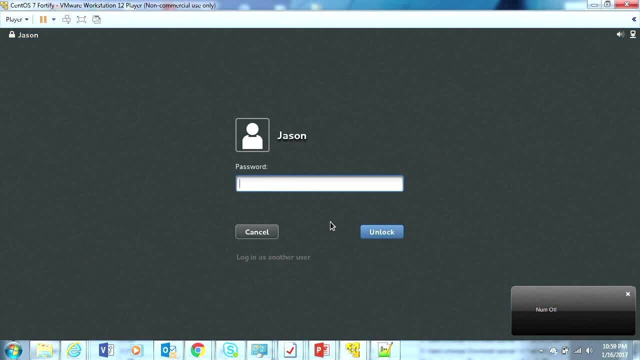 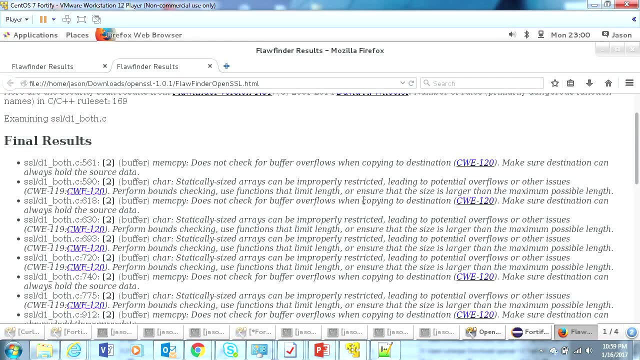 So over here is a tool called FlawFinder. Again, it works in a very similar fashion. It's primarily for C C++ code. It was written by David Wheeler I mentioned earlier, And it gives you something. It's organized by the common weakness. 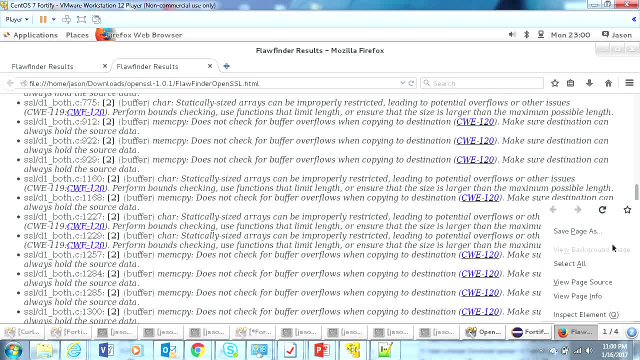 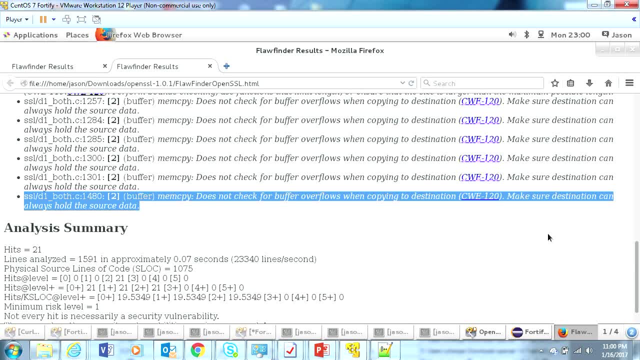 that it's associated with And again, I believe this also identifies that particular buffer file. But one thing: it doesn't know, if it's looking at a particular file, whether you're doing sanitation somewhere else in the program. So that's kind of a weakness of this style of detection tools. 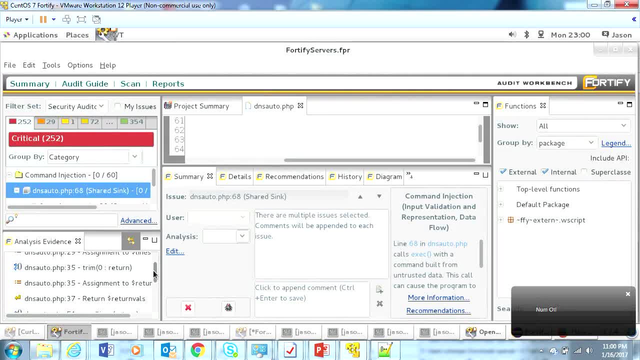 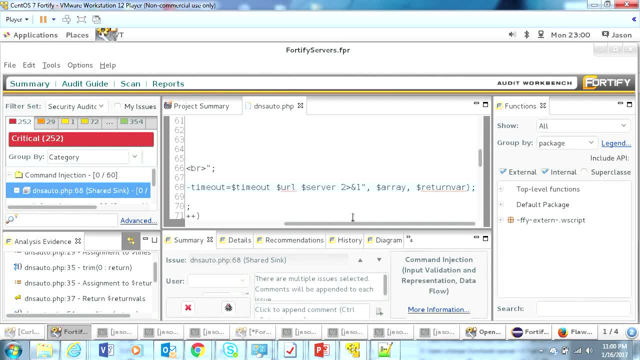 On the other hand, if you have something like this, a commercial tool called Fortify, it injects itself. It injects itself into the compilation project for compiled code And it does a more detailed flow through the entire application. It tries to at least. 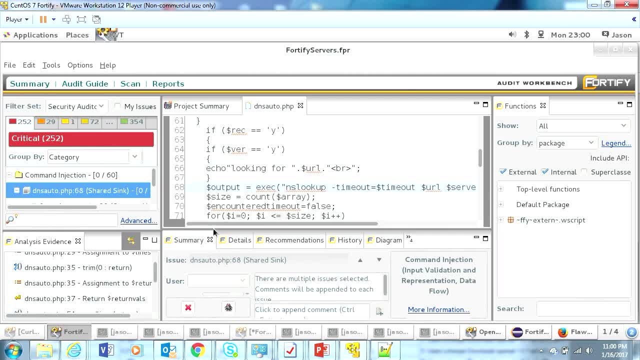 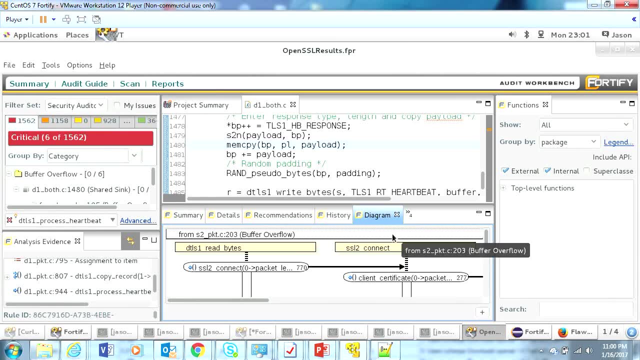 And again it detects the issue. Oh, this is a sorry Hold on a sec. Yeah, this is the OpenSSL vulnerability detected by Fortify. I wouldn't have done this before that was released. In all fairness, they did add some better heuristics. 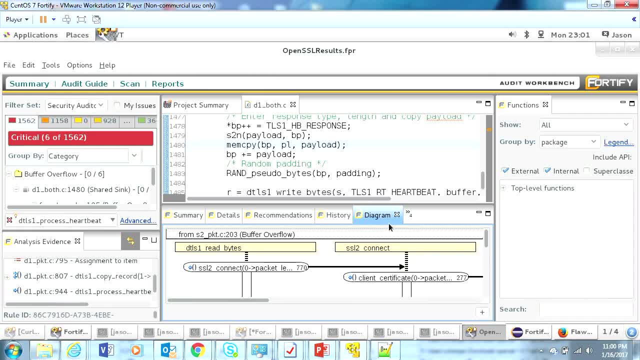 to try to detect this. What I really like about this is that, again, it's a lot easier. This it breaks down a nice little diagram too, so you can help trace back where the tank came from. One thing you will note: it found quite a few other. 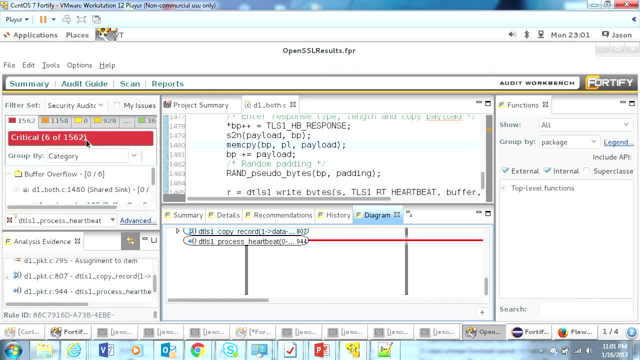 vulnerabilities in the code And you would be hard pressed to go through each of these and determine if they're real vulnerabilities or not. But certainly could be some other ones out there waiting to be found. All right, OK. Well, I'm out of time. 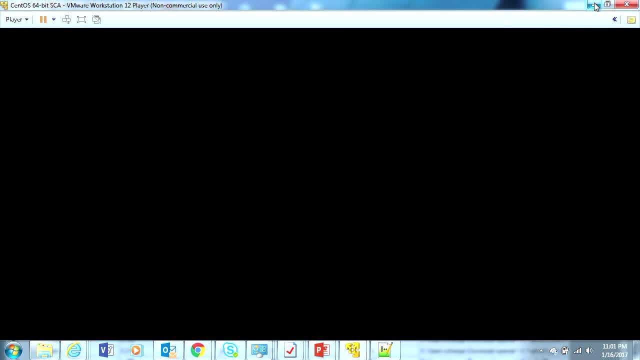 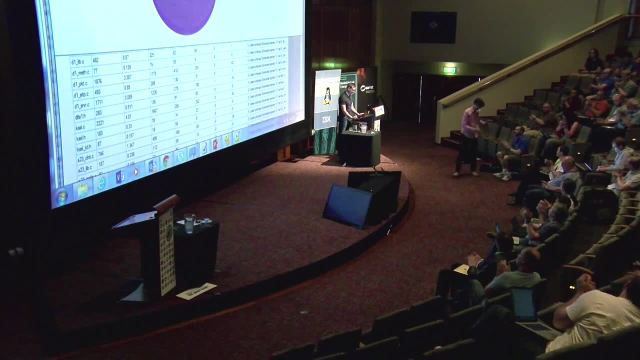 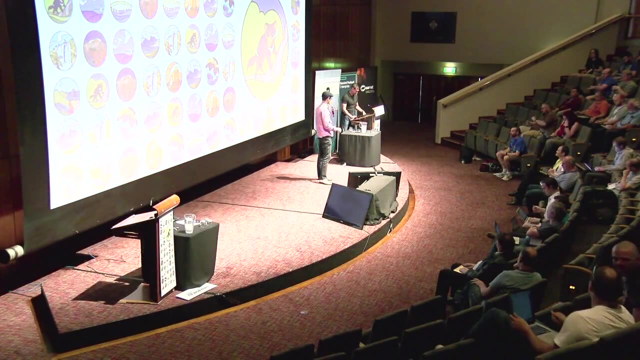 I was going to show you another one, But you get the idea, I think. If you have any questions, feel free to approach me, And thanks again. Thank you very much, Jason, for that secure development tour de force. It's now afternoon tea after afternoon tea. 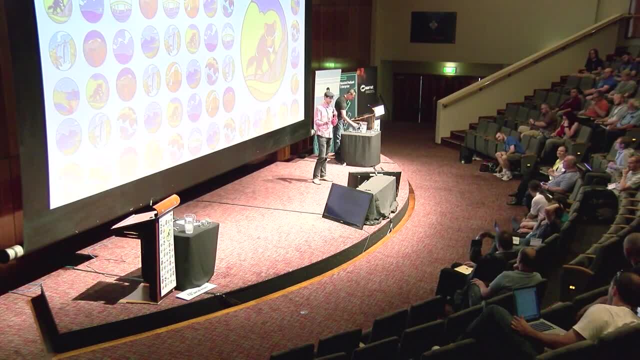 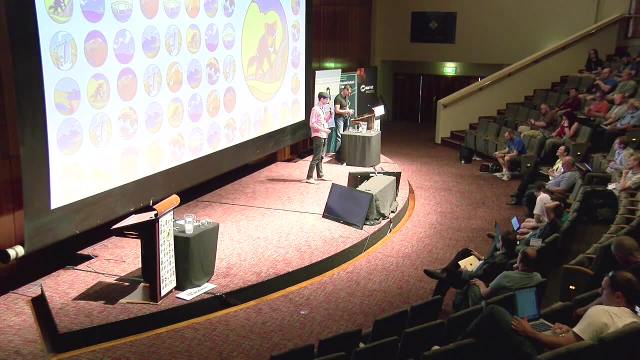 in our final session. Up first we have Christopher Biggs giving a talk on IoT security, the internet of scary things And talking of scary things. after that is a talk on internet ghosts And after that I'll be doing a very quick free IPA project.